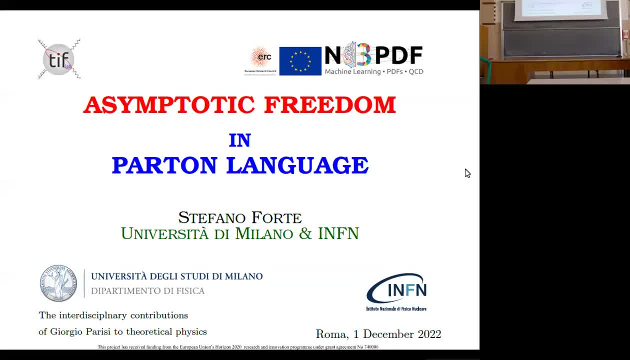 Okay, I think we can start, So welcome everybody to this seminar. This is the fourth seminar of this series dedicated to the many contributions of Giorgio Parisi to theoretical physics, And it is also the last seminar of the year, so we will start again next year in February. so we will have another 10 seminars next year. 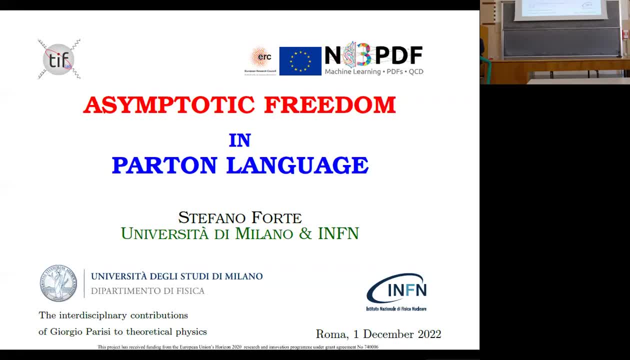 The topic today is QCD, the theory of strong interactions and in particular it's perturbative QCD. We will also have some other a couple of seminars on non-perturbative aspects of QCD next year. So, as you know, we have selected the topics by looking at the most cited paper by Giorgio, and this is one of these most cited papers: Asymptotic Freedom in Parton Language, which was written in: 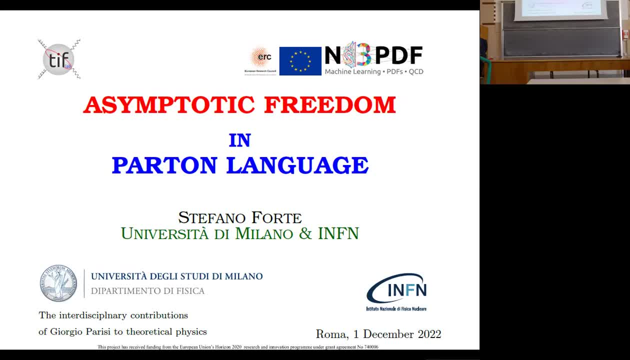 1977 with Guido Altarelli who sadly passed away a few years ago, And it is actually one of probably one of the most well-known papers in particle physics in the high energy physics community. It counts almost 8,000 citations on the INSPIRE database and I've checked yesterday and if I sort the papers on the database by the number of citations and I removed the PDG. 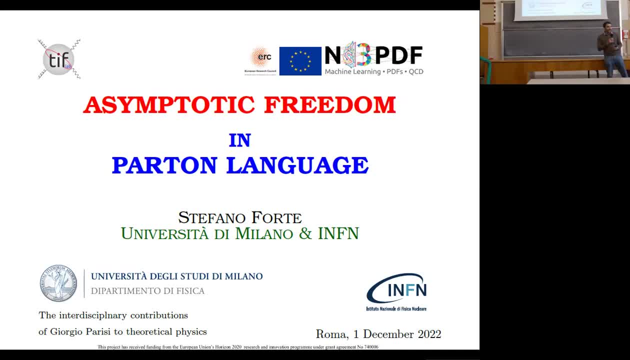 And the big experimental papers. it is number 11, so it's really remarkable. It's the 11th most cited papers in particle physics of all times. But you know, the contributions of Giorgio to QCD are not restricted to this only paper. there are several others and this will be subject of the seminar today. 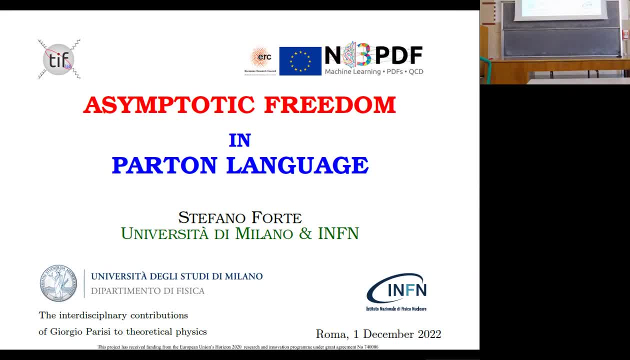 And the speaker that we have is Stefano Forte. It's really a pleasure to have you here. Stefano is full professor at the University of Milano Statale. He came from Turin where he studied undergraduate, where he was an undergraduate student, and then he moved to MIT under the supervision of Roman Jakiv. 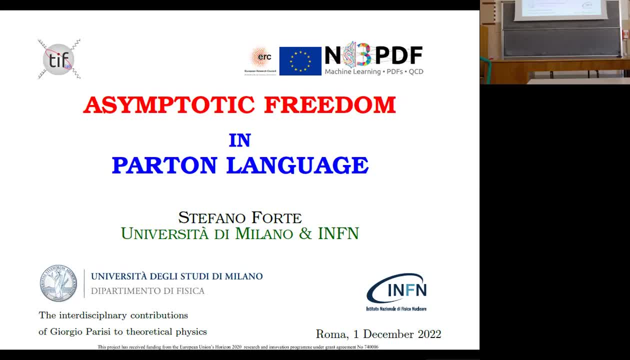 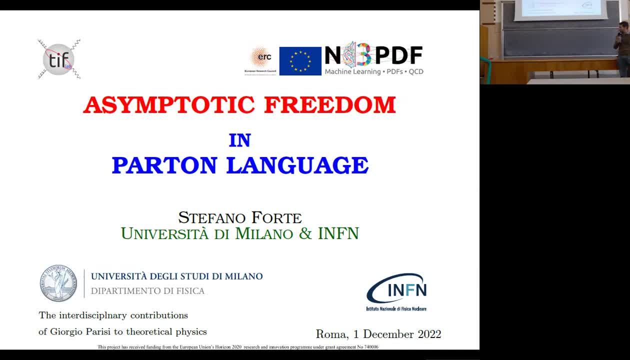 Stefano is a renowned expert on QCD and one of his main activities nowadays is the determination of part and distribution functions, which are intimately connected with the topic of this paper, and he's the leader of the NNPDF collaboration who revolutionized, I would say, I think, the way PDFs are determined from data by using machine learning techniques. Stefano is an expert on QCD and one of the main activities nowadays is the determination of part and distribution functions, which are intimately connected with the topic of this paper, and he's the leader of the NNPDF collaboration who revolutionized, I would say, the way PDFs are determined from data by using machine learning techniques. 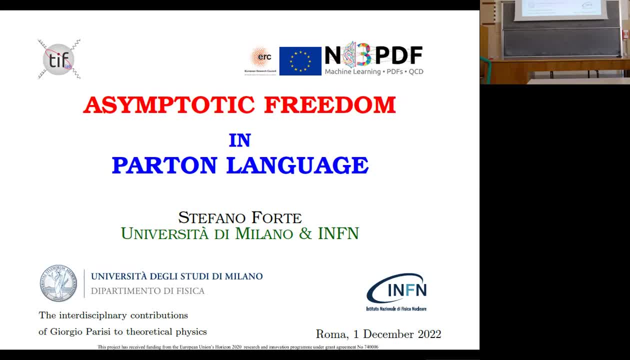 Stefano is also involved in many activities of the high energy physics community, but I don't want to steal more time. I think you can start your seminar, so thanks very much for being here and you can start. Okay. thank you very much. 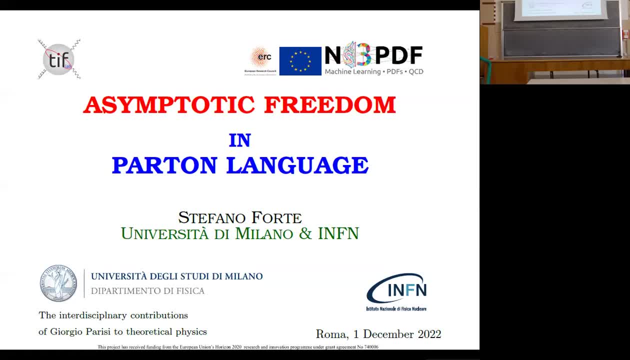 Thanks. Thanks, Marco, for this lavish introduction. So the paper that gives the title to my talk today is actually the culmination of a number of papers of developments of which Giorgio has been an author. This does not seem to work, Okay. yeah, I guess what we had to do was kind of get unstuck the slides Right. so it's a 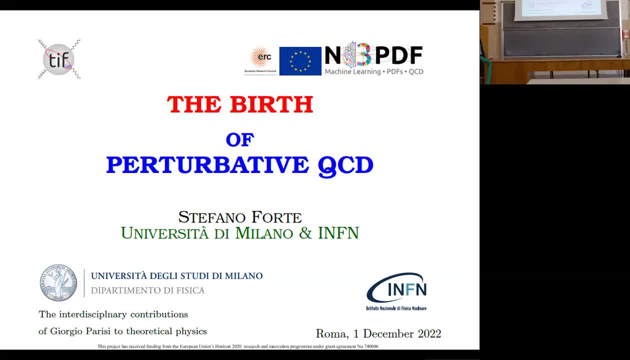 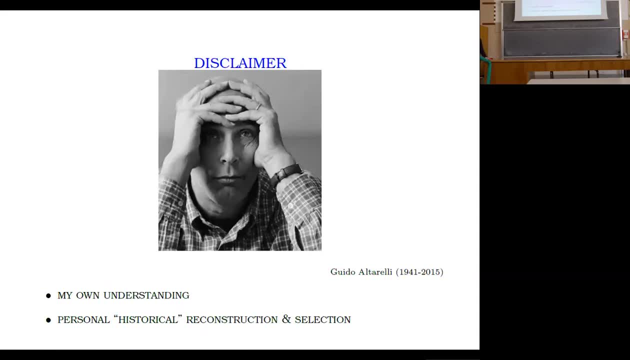 culmination of a number of papers that are really at the heart of the development of what is modern perturbative QCD. And I guess I should start with a disclaimer, which is the following: I mean, I realize that most of the talks in this series are given either. 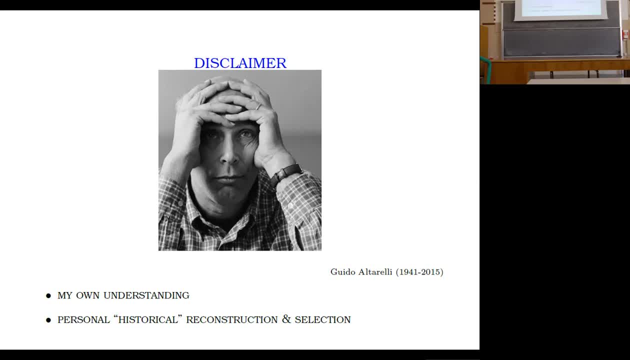 by co-authors of Giorgio on the paper or on, you know, very closely related topics. I'm sure that in this case, the co-author of the paper that gives the name to the talk would have given a much better talk than mine, not just because obviously he knew, you know he had. 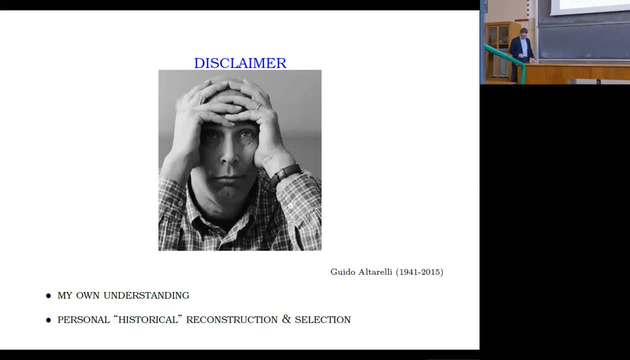 an insider view, but also in terms of science. Now, even though I spent a very large number of hours discussing with Guido, we actually never talked about this paper, or indeed his old papers, because Guido did not like to talk about. 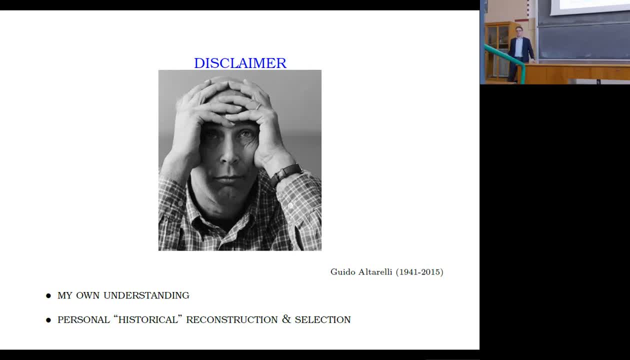 the past. So the disclaimer is the following: that I of course know very well the paper with the Autorelli-Parisi equation, which I studied as a student, even though I was a PhD student. about 10 years after the paper was written, it was already a. 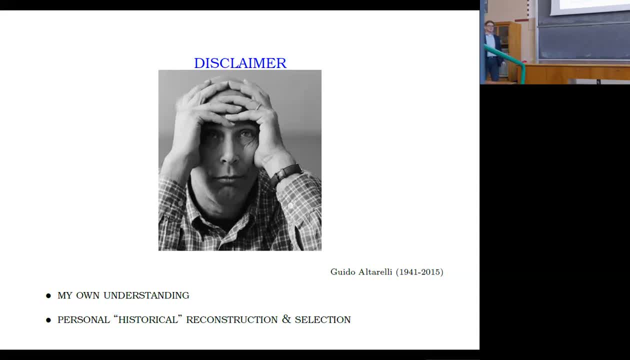 classic. I knew several more papers by Giorgio that are related to this line of thought- but you know I don't have an insider view- and many more papers I actually discovered over the last several weeks as I was preparing today's talk. So you know what I'm trying to, what I will try. 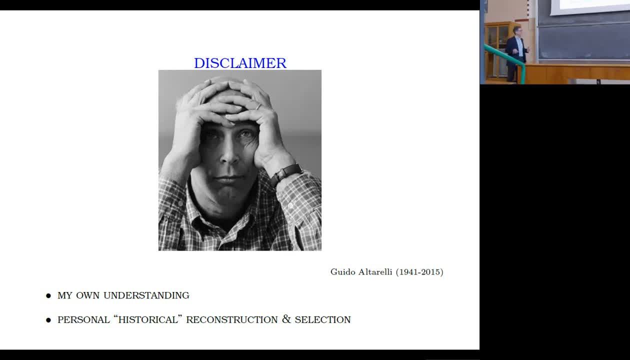 to give is some kind of, you know, personal reconstruction of the line of thought which is behind these developments. and I'm, of course, very honored to have Giorgio sitting in the front row and you know, I thank you for this invitation and you know, I hope that I'm not going to say: 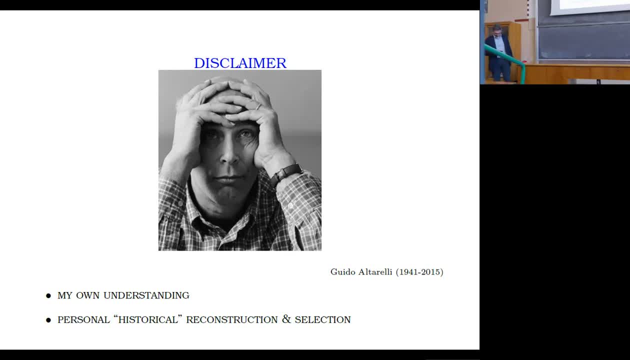 anything silly And if I do, you know I'd be grateful for. to Giorgio, for you know corrections or you know telling me what I misunderstood or I got wrong. Now, the contributions of Giorgio to perturbative 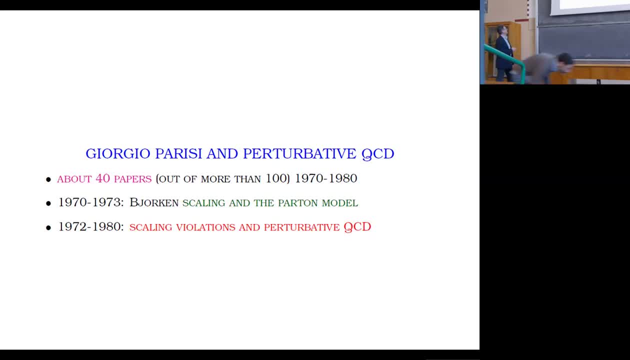 QCD are very numerous and they are concentrated in a very short span of time. They are all written between 1970 and 1980.. If I define, you know perturbative QCD in the narrow way, so not including. 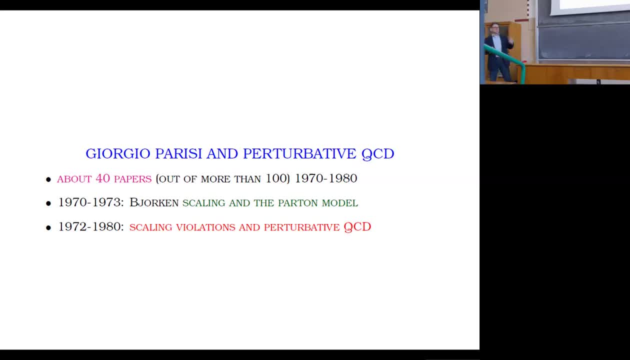 lattice, not perturbative QCD, but perturbative QCD in the narrow way. so not including lattice, not including subsequent non-perturbative developments. it's about 40 papers out of more than 100 that Giorgio wrote using these years and you know they can more or less. 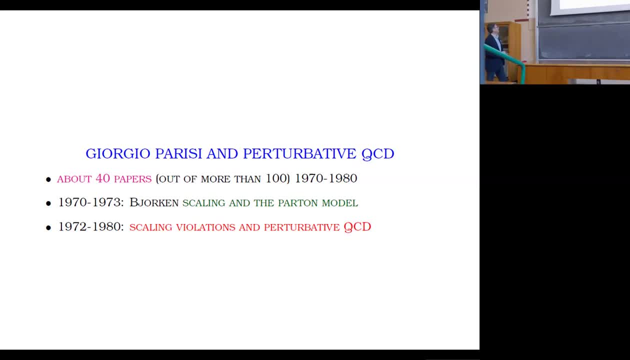 be grouped into broad categories: A number of papers written in the early 70s which have to do with understanding Birkin scaling and the Parton model, and then a larger number of papers written in the rest of the decade and partly overlapping with these. 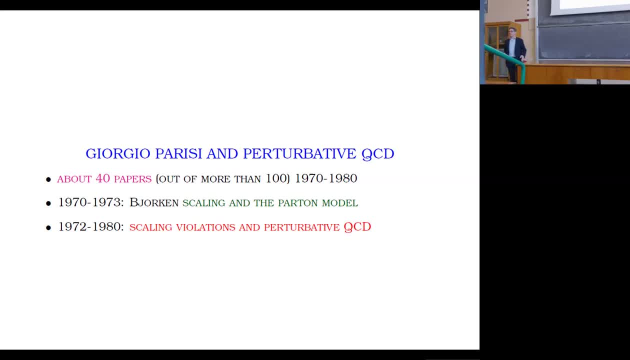 that have to do with understanding scaling violations and which, indeed, are the ones that lead to perturbative QCD. And you know, when you look at these papers, you know looking at these papers in the last several weeks, one thing that struck me is that often people have the impression 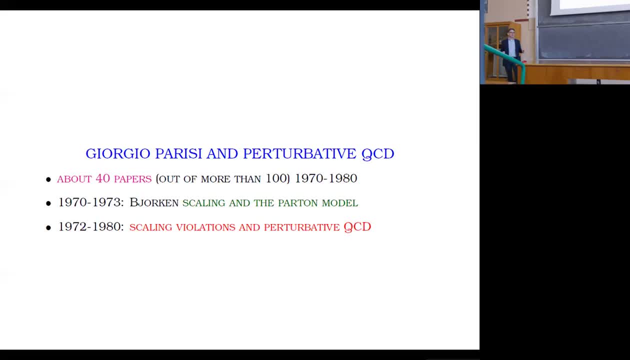 that the standard model was mostly born and developed on the other side of the ocean. And you know it's quite a bit of a, And you know it's quite a bit of a And you know it's quite a bit of a. 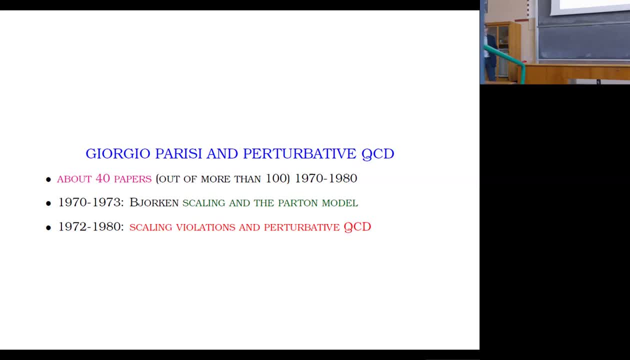 clear once you look at this that this is absolutely not the case. I mean not just the Eltrali-Paris equation, but there is a number of things that clearly were developed either here or in Paris or in other European institutions where Giorgio and his collaborators 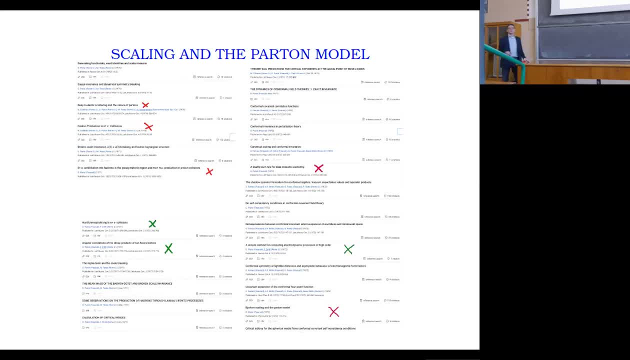 were working. Now, just to give an impression of the papers having to do with this first set of topics related to the Parton models I'm showing here. you know it's very small, but it's just to give a get a visual. 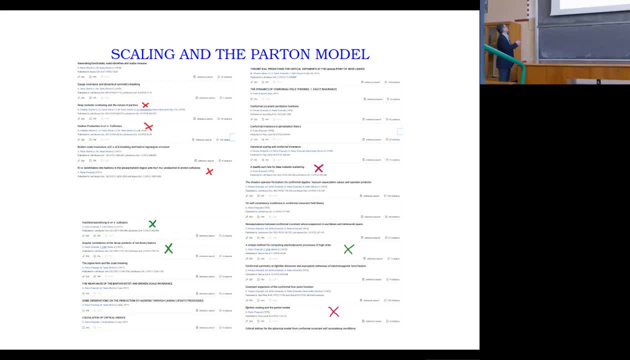 impression is the list of papers that Giorgio wrote from the very beginning, downloaded from spires up to well, I mean I guess the first 30 or 40,. the Red Cross is perturbed with QCD papers. the Green Cross, it's actually QED papers which, however, introduce techniques. 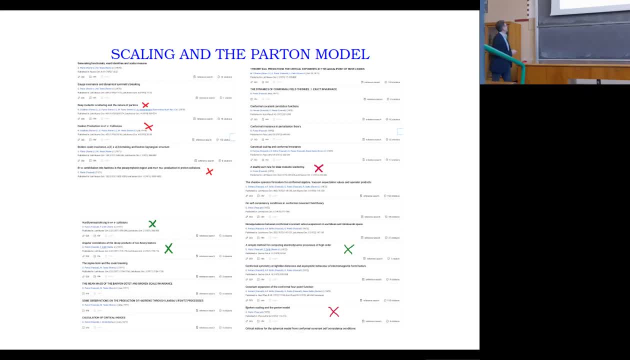 that will be relevant for subsequent QCD developments. And then you know. you can check out the titles of other pieces of work. Many of these papers have to do with conformal embrace variance, conformal field theory, calculations of critical indices. so that's really statistical. 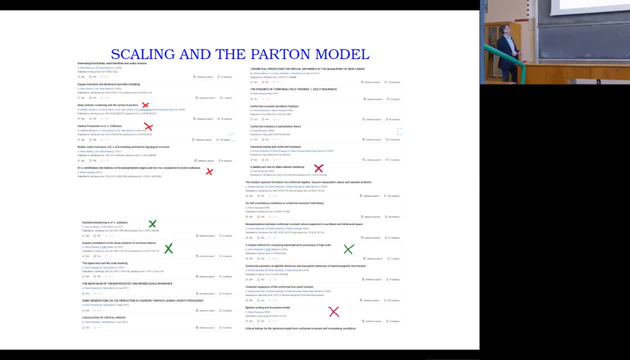 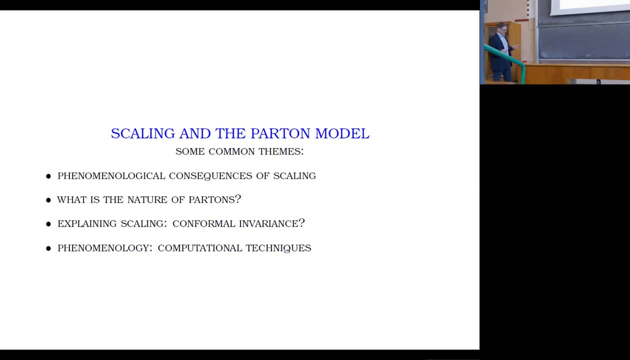 mechanics, But you can see that the Parton model and QCD play a dominant role, And these papers have a set of common themes that are mostly related to the desire of understanding the phenomenological consequences of the theory that was being developed. So, as we shall see, 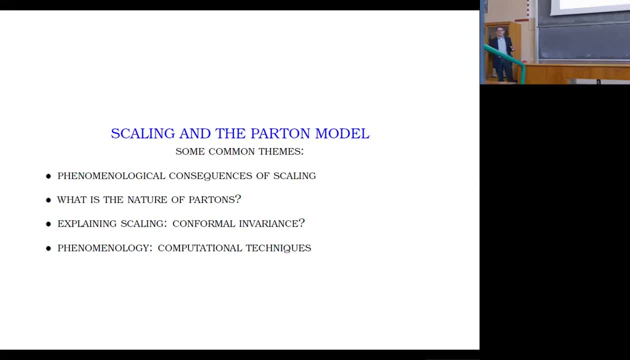 in the remainder of the talk. many of the ideas that happened, at least as I see them by reading the papers- were something that comes from an actual desire of being able to tell, by looking at the data, what's actually happened. So you know, first set of papers has to do with the 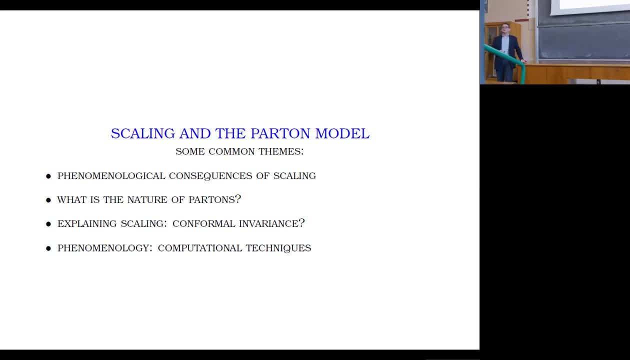 phenomenological consequences of scaling, and then understanding what is the nature of Partons, which, as I'm going to say in a few minutes, was not at all obvious at the time, and then explaining the origin of scaling, possibly with conformal invariance, which is related to the other subject that Giorgio was working on at the 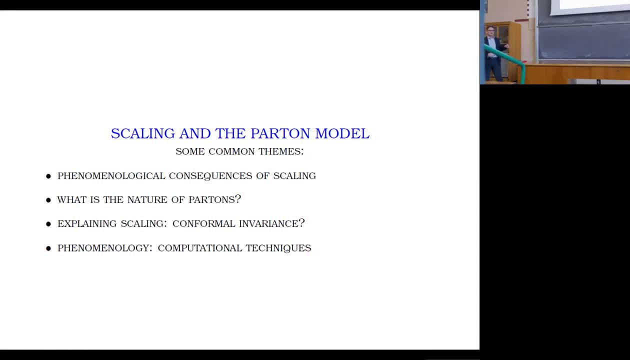 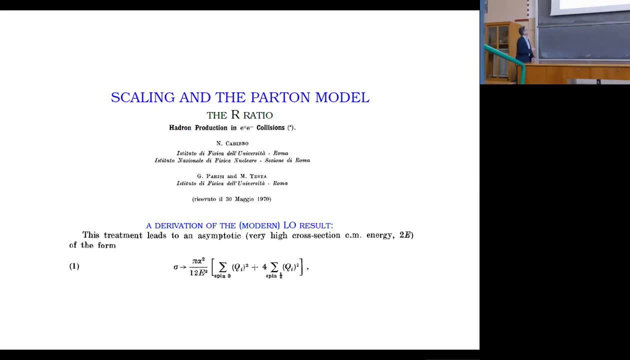 time, and then developing computational techniques- And on this, you know, I at least had a surprise, discovering some developments again, as we shall see Now. this is the earliest paper that Giorgio wrote on perturbative QCD. It's called Hadron Production in E plus E minus Collisions. 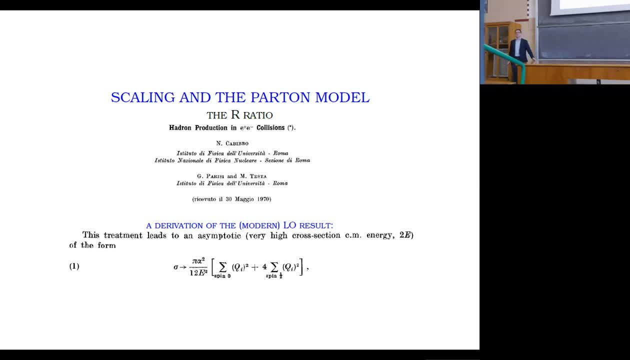 Of course, Giorgio was working in Frascati, where the Adone you know, E plus, E minus- Collider was actually collecting data. So that was something that was real And this, you know, this paper, presents what we currently teach to students as the 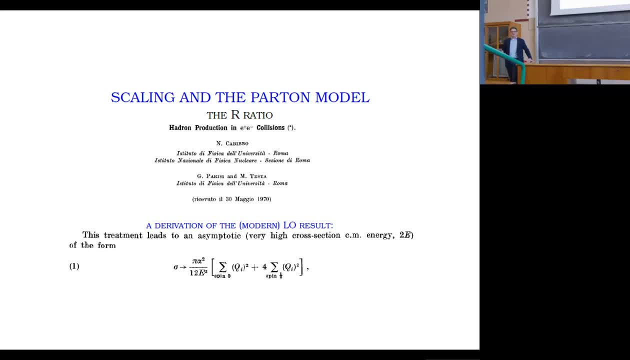 computation of the R-ratio, the ratio of the cross-section for total cross-section for producing Hadrons divided by muons in E plus E minus collisions, And you know, the paper gives right away the result, which is of course, again the result, the leading order. 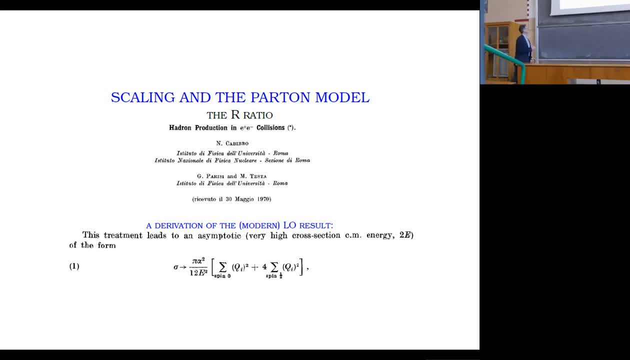 the result we teach to student, which is the sum of the square of the electric charges of partons, except that the only thing which is maybe unusual here is that there are both spin zero and spin half-charged partons, which of course you know we have. you know, which is something which? 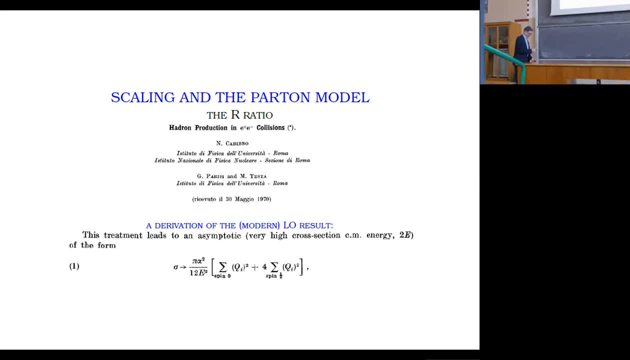 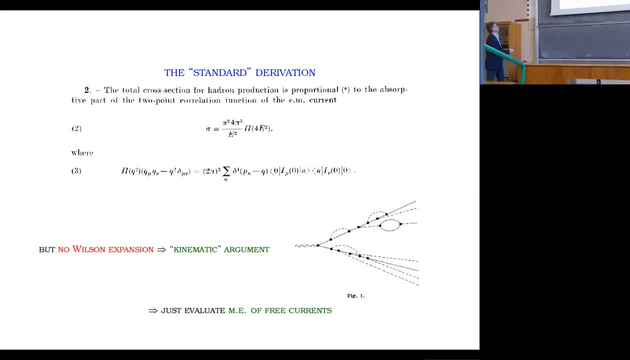 we don't have now, and it is related to the fact that at the time it was not at all clear what partons are. Now, the way this result is derived is actually quite clear. It's not just that. it's quite interesting because the way the calculation starts is exactly the same way you find in you. 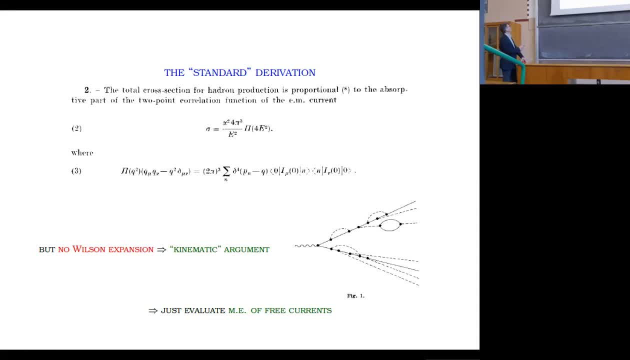 know Peskin's textbook. I mean you start by writing the cross-section in terms of a two-point correlation function of the electromagnetic current, and then you say you get it from the imaginary part, from the absorptive part, And you know the way we would do it in modern language is: 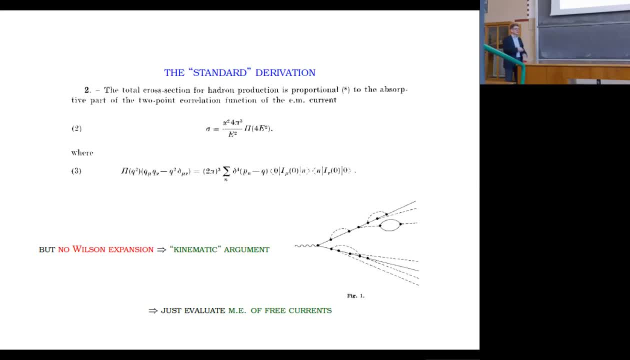 you then use the Wilson expansion and then you say the dominant operator is the vacuum and then you go and calculate vacuum polarization and so on. But here you know the Wilson expansion was being born at this time. It was clearly not a usual tool. 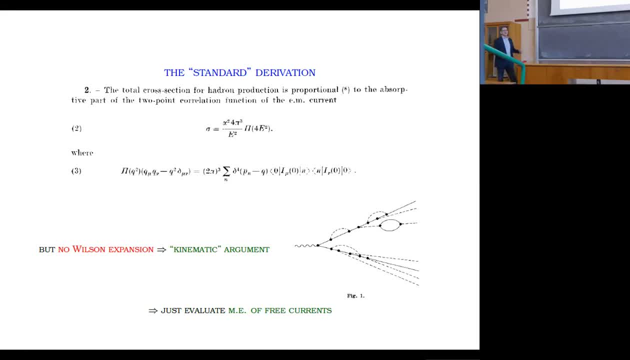 So a kinematic argument is used instead. The kinematic argument is that hadrons are produced mostly as a pair of back-to-back jets. These jets do not talk to each other. There is no at high energy, there is no PT transfer between them and therefore you can actually calculate. 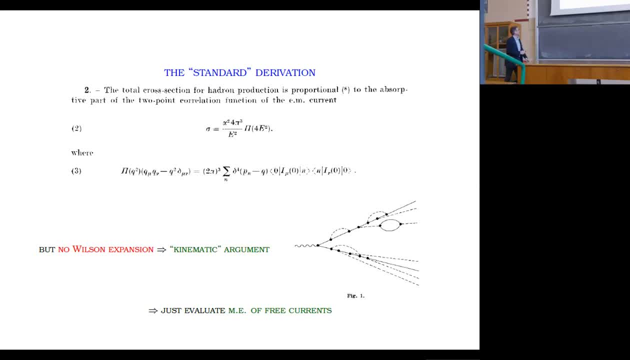 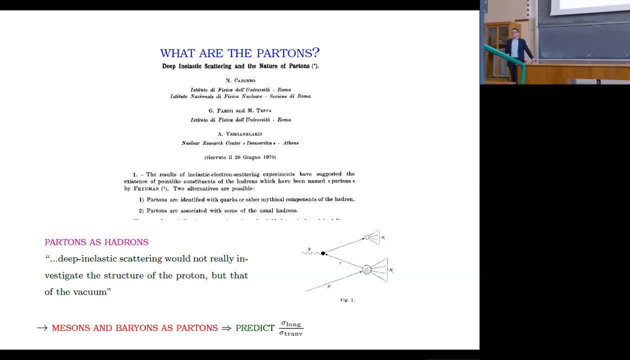 the two-point function as if it were the matrix element. Now, as I said, the nature of partons or what partons are was not at all clear at the time, And in fact there is a number of papers, including the one which I'm showing here. 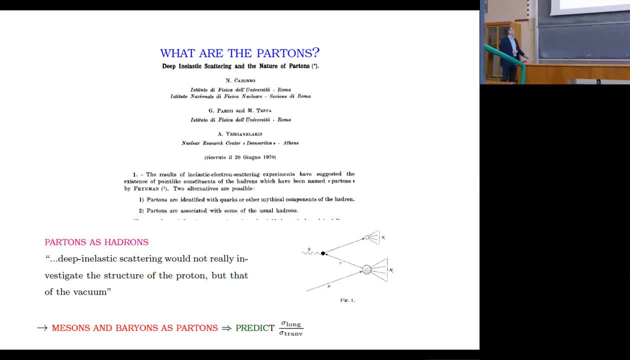 which have to do with asking the question: can we actually tell what partons are? And you know this paper starts with an interesting sentence, which is: you know there are two possibilities. Partons are identified with quarks or other mythical constituents of the. 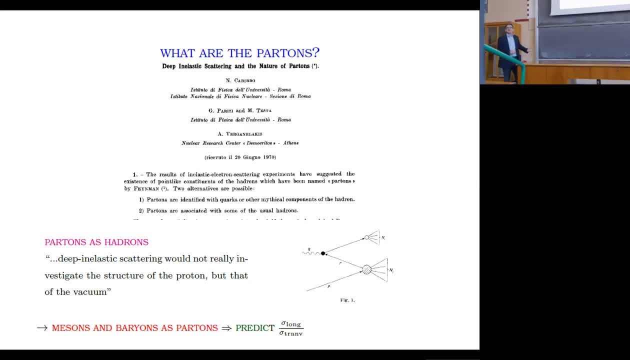 hadrons or else partons are, you know, not identified with quarks, And you know there are actually, you know, mesons and variants, And the paper here was then taking the point of view that the latter possibility should be taken seriously. And then, if so, you know, if partons 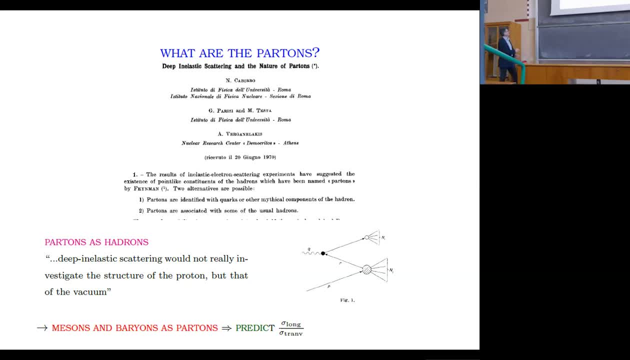 are hadrons, then deep dynastic scattering would not involve the structure of the proton, because the idea is that a virtual incoming photon produces, you know, hadron-anti-hadron pair which then interacts with the proton. But the interesting thing is that then you know, 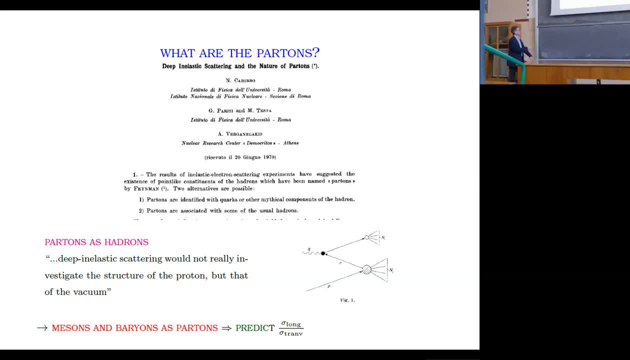 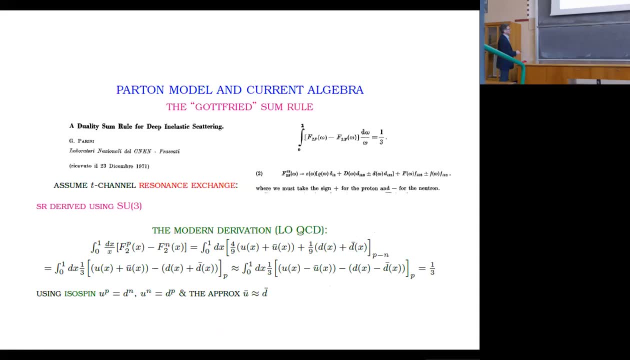 making this hypothesis, one can actually calculate predictions, for example for the ratio of longitudinal to transverse cross-sections, which allows you to tell which is the case Now. interestingly, some of the parton model results that were derived by Georgia at this time are now considered to be: 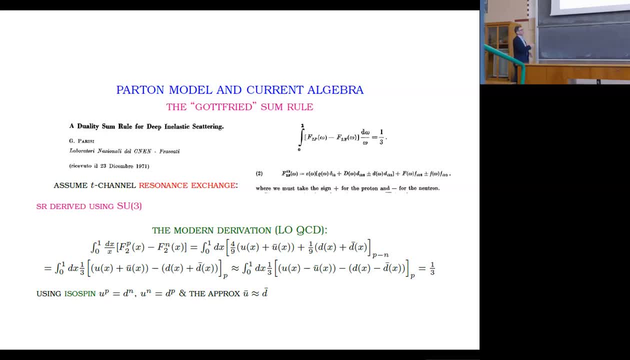 classic parton model results. One is what is normally called these days a Gottfried sum rule, which is derived in this single author paper as a duality sum rule. So it's derived. so the sum rule is the, the integral of the first moment of the proton minus neutron structure function, which is equal. 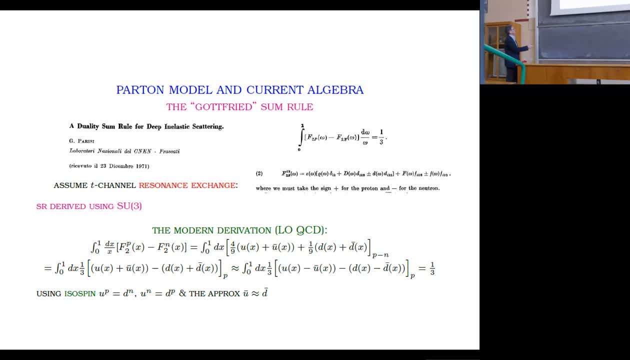 to a third. The modern derivation in leading order, QCD, is based on using isospin, which says that the number of up quarks, so that the up quark distribution in the proton is equal to the down quark distribution of the neutron, And conversely, and also making an approximate SU2 symmetric. 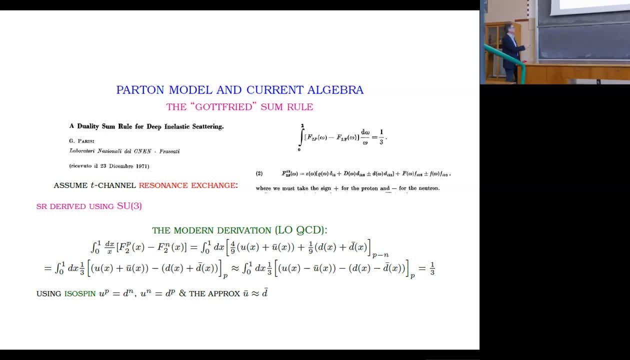 hypothesis for the nucleon C, which now we know not to be fully correct but rather to be violated. But you know, this derivation was standard until maybe 15, 20 years ago, when people started seeing deviations In this paper instead. the result: 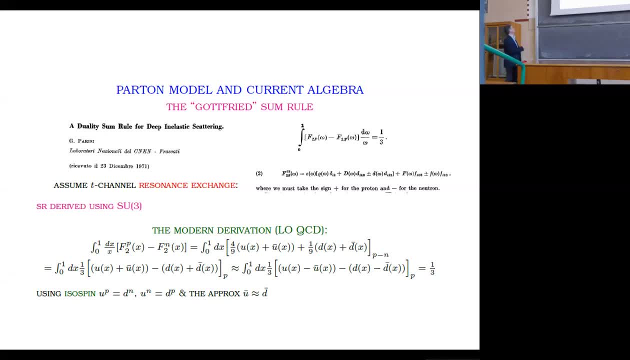 is actually derived without using directly a parton picture, by assuming that the deep gnostic scattering process is dominated by T-channel resonance exchange, so that the structure function are written as a sum of resonance contribution, which are in fact classified with F and D, SU3 couplings, singlet and octet. 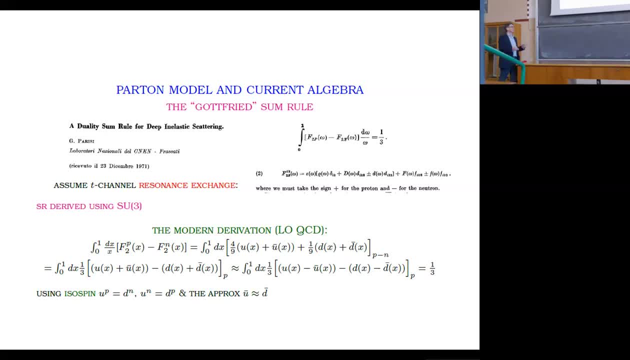 You know, with a plus sign for the proton and a minus sign for the neutron, for the SU3. SU2 once, and then using SU3 symmetry, which produces the same result that we get today, which is driven by, indeed, SU2 symmetry. 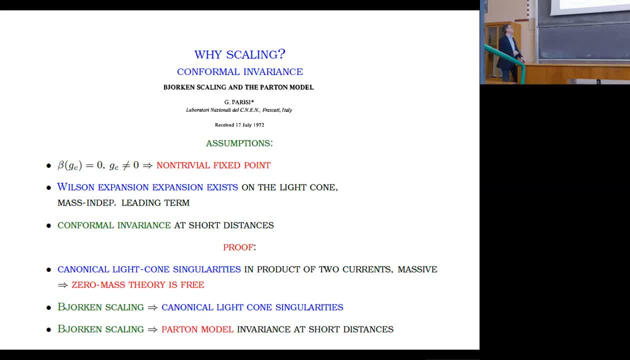 As I said, a major line of development at this time was trying to understand what is the origin of the Bjerken scaling, And the natural hypothesis was that scaling might be related to scaling variance of the underlying theory. So, for example, in this paper from 1972, what Giorgio does is make a number of assumptions. 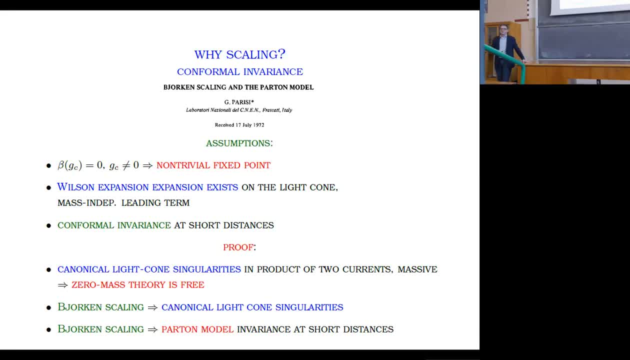 which are basically related to the existence of a non-trivial fixed point of the beta function of QCD, from which one then derives a proof which is based on the following syllogism that you know: canonical light cone singularities imply that the zero-mass theory is free. 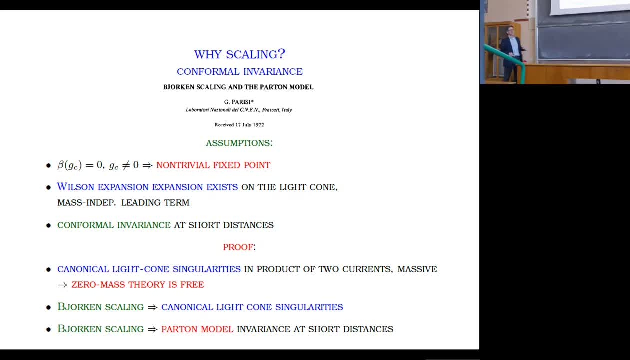 but Bjerken scaling implies canonical light, cone, singularities and products of currents. so Bjerken scaling implies that the zero-mass theory is free. so the Parton model at short distances, which is, you know, an interesting possibility, which turned out not to be what. 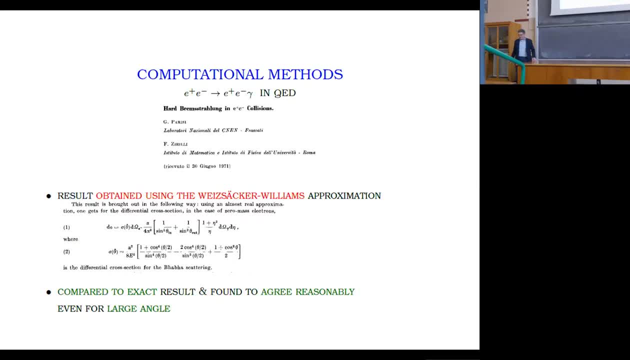 actually happens, but was natural enough at the time. So I mentioned that some of the papers written at this time were actually QED rather than QCD, And I'd like to mention one or two which are which I found remarkable. I didn't know. 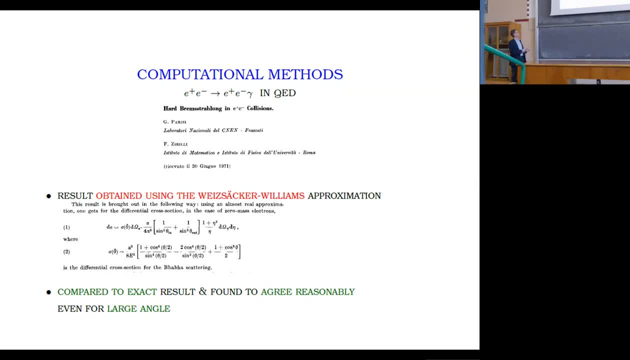 of them because of the techniques they introduce. So the first of these two papers is a computation of photon radiation in E plus E minus, so the process E plus E minus, going into E plus E minus gamma, which is actually computed. 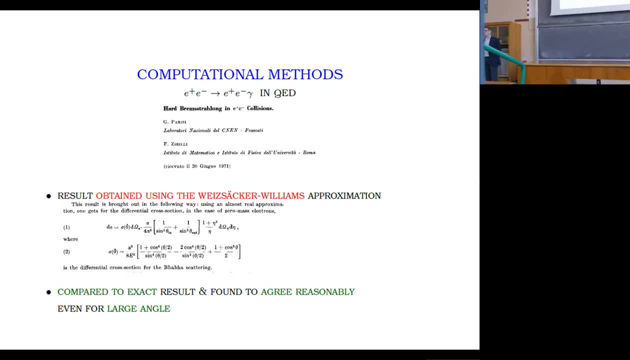 using the Weizsäcker-Williams approximation, which has, I guess, most people or many people in the audience know and, as we are going to see, will play an important role in the Altarelli-Parisi paper. And then the result found using Weizsäcker-Williams is compared to the exact result and it's 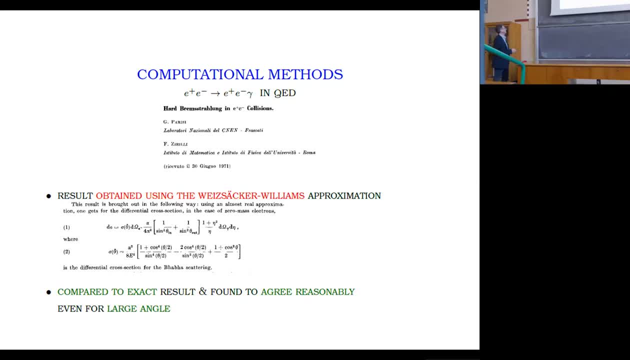 surprisingly found to agree with it, even in the region of large-angle photon scattering, while Weizsäcker-Williams would only hold, should only hold for small transfer of momentum. But then the really interesting thing which I discovered is the way, the exact calculation. 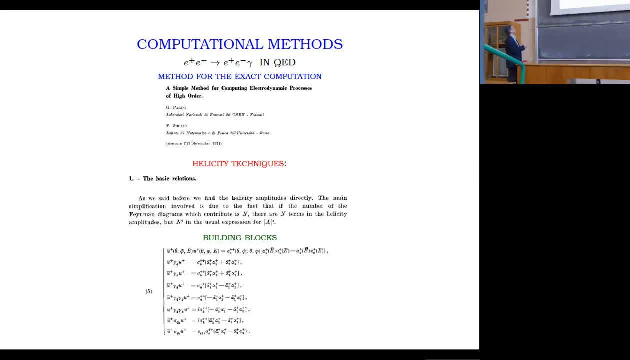 is done. So the exact calculation is presented in a In a different paper, where the following interesting statement is made: we find the helicity amplitudes directly. The main simplification is due to the fact that if the number of Feynman diagrams, which 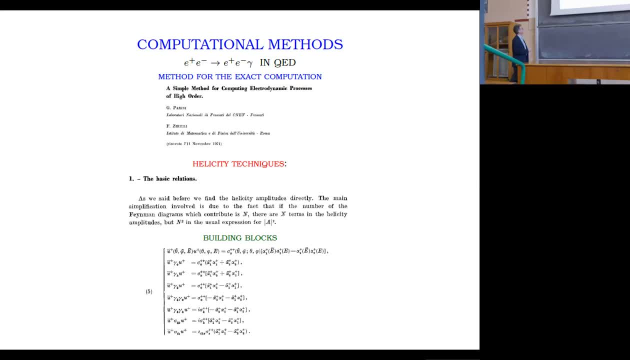 contribute is n. there are n terms in the helicity amplitudes but n squared in the usual expression for a squared, and then you get a list, of you know formula which has what we would call in present day Mangano-Park formula. 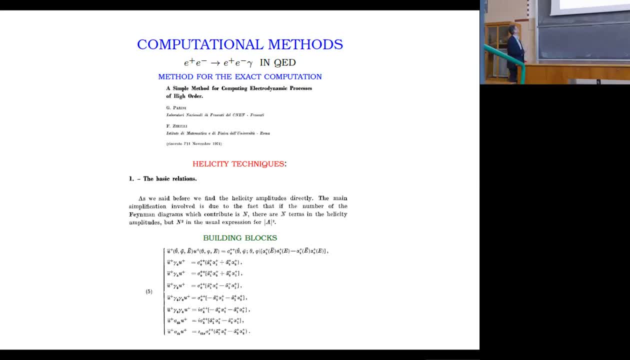 So you know, maybe if Giorgio had Kept working on this, we would have had the helicity formalism in the 1970s instead of having to wait until the 2010s. but okay, that's not the way history happened, but still. 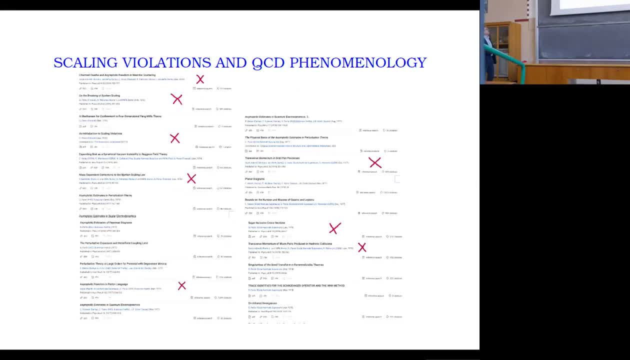 I found this development remarkable. Now this brings me to the subsequent line of development Here. I'm not even trying to show you all the paper, I just show you a snapshot of some of the papers which were written around. asymptotic freedom in Parton language. 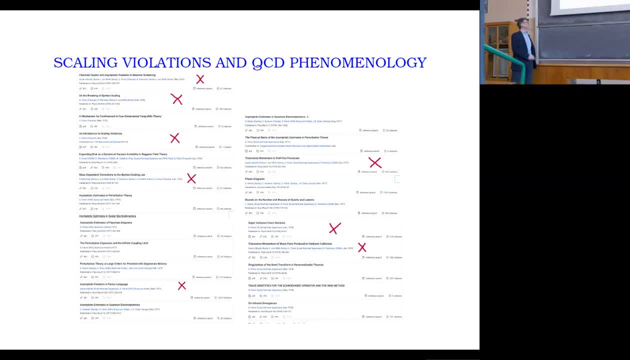 Still the fraction. Some of the red papers- so you know QCD papers- is striking. It's maybe half of them. The other topics that Giorgio was working on started being more diverse. There are many papers that have to do with the high-order behavior of perturbation theory. 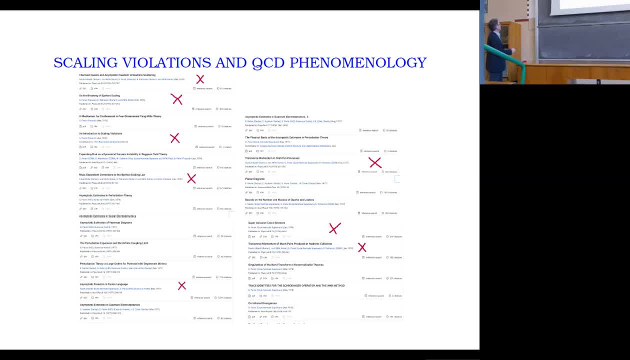 which I'm going to mention briefly at the end of my talk. so you know: asymptotic estimates in quantum electrodynamics, asymptotic estimates in theory with fermions. there are many papers about. There started being papers about non-perturbative methods, but still an important focus is on 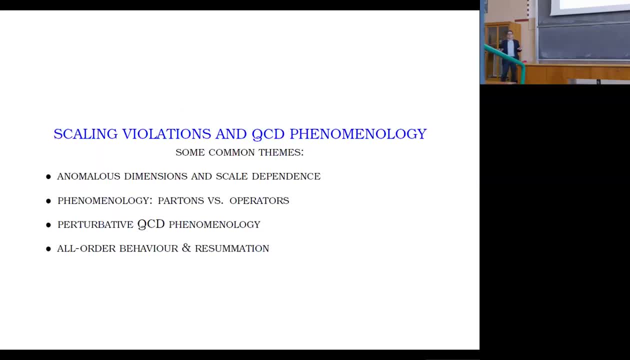 perturbative QCD. Now, the common themes of this line of thought that occupied Giorgio for the best part of the decade is understanding the violations of scaling, so understanding anomalous dimensions and scale dependence, And again trying to. 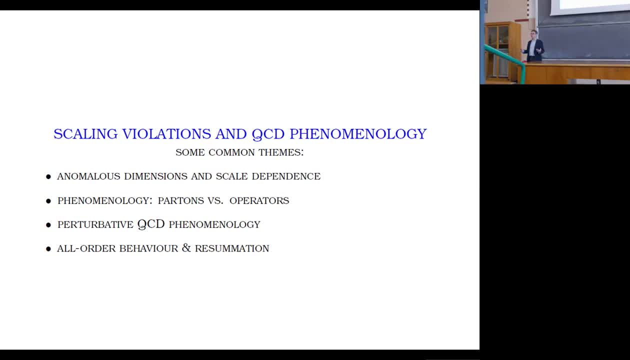 Relate the then-dominant formalism of OPE Wilson expansion to something closer to the data, So something closer to you know, Feynman diagrams that correspond to the processes you actually see in the lab. And then, once this program was accomplished, through the Altarelli-Parisi paper, trying 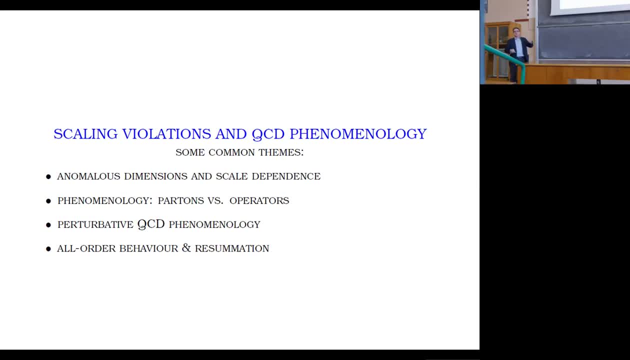 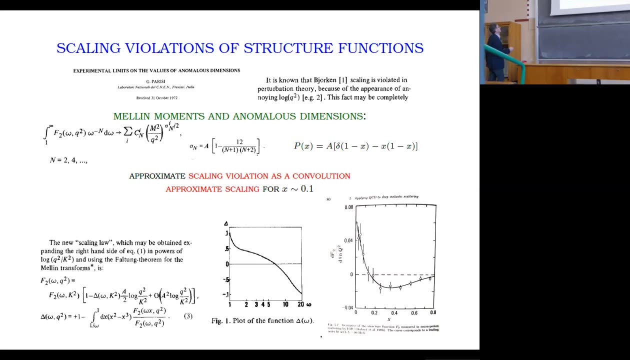 to follow some of the perturbative QCD phenomenology and then trying to push the theory further by looking at all-order behavior, And you know the birth of what is modern QCD, or estimation. Now, the first paper that Giorgio wrote, or at least the one that I found about scaling, 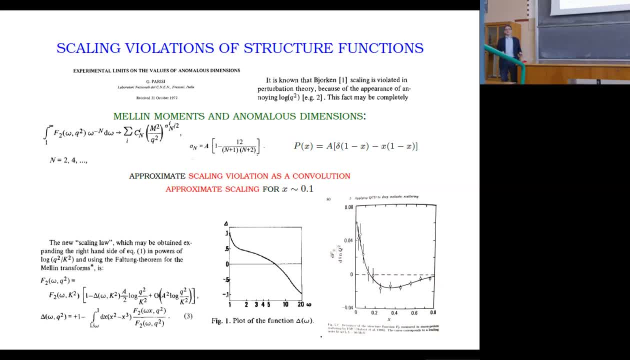 violations is a paper which is quite early- 72, so it overlaps with the time when he was still thinking about the arcane scaling. And you know the paper, which is again single author- Experimental Limits on the Values of Anomalous Dimensions- starts with this striking sentence. 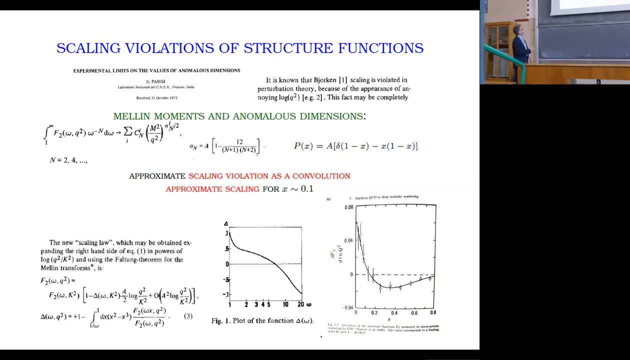 It says So in this striking sentence. it is known that the arcane scaling is violated because of the appearance of annoying logs of Q-square. And then you know, one tries to show how the annoying logs of Q-square appear, and 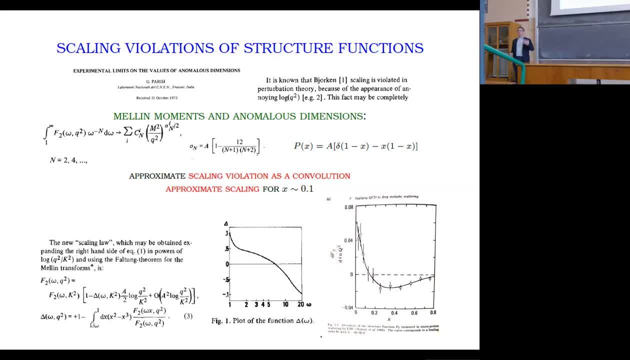 you know, this is the first time, at least, that I saw the modern Mellon moment formalism showing up. So the idea is, if you're right, if you look at the Mellon moments of structure, functions or of part and distributions instead of looking at the physical momentum spectrum, you're 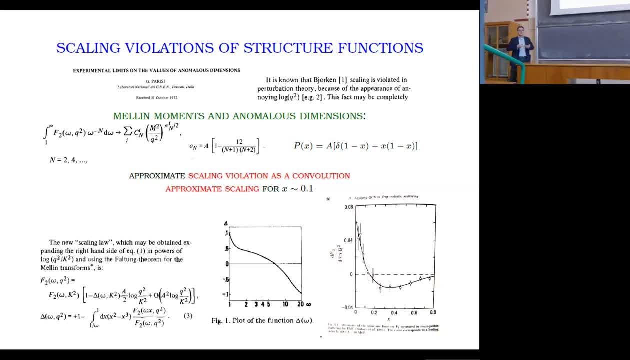 looking at the physical momentum space, then you realize that they have a very simple decoupled Q-square dependence. They depend on scale, as the scale raised to some power or, if you prefer, as the exponential of an anomalous dimension times the log of the scale itself. 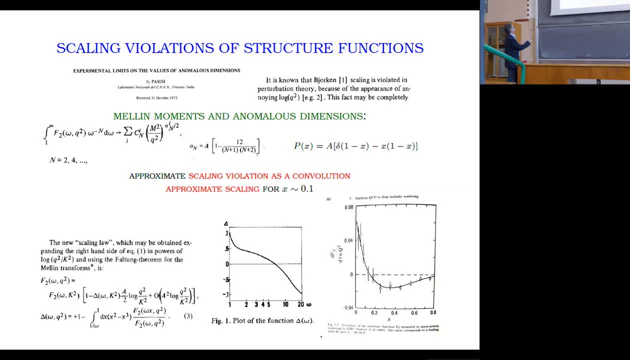 So the logs of the scale exponentiate and the coefficient of the exponentiation is given by an anomalous dimension. Now this paper is still related to trying to understand the arcane scaling. So why do we see scaling, Despite the fact? 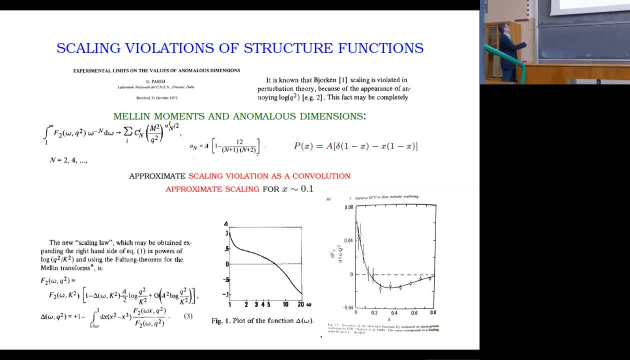 The scaling is violated and it suggests the following idea. So the paper is based on having an ansatz for the anomalous dimension which is written here, So it's a kind of guess. This guess can be viewed as the Mellon transform of some function which I wrote here and 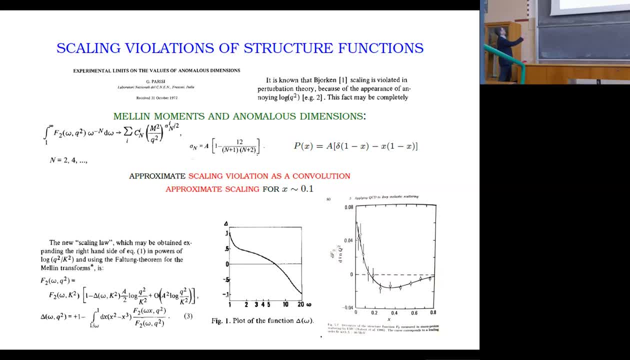 then one notices that if the moments of the structure function behave like this, then this means that the structure function itself behaves in a way which is shown here. So it is driven by the behavior of this function here. And then, if one looks at the way, 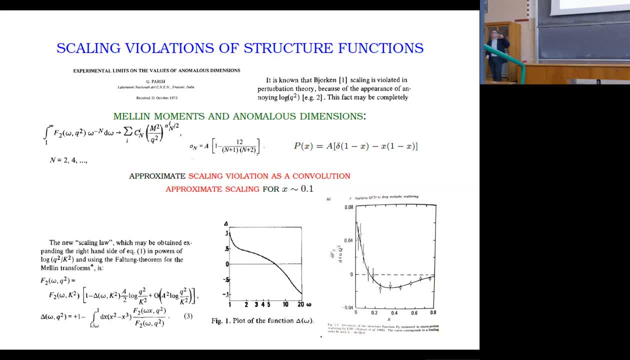 So omega here is 1 over x, where x is the arcane, x the fraction of the momentum carried by the partons, And if one then looks at the scale it depends. in this equation one finds that it has a shape like this: 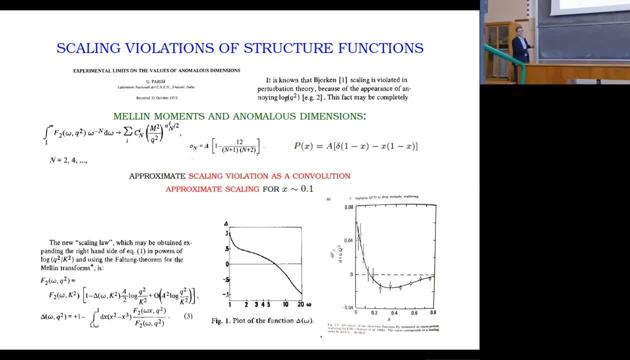 So it changes sign, which means that if one is sitting for actual data in the region of 1 over x equals 10, so x equals 0.1,, then the function has a zero and there is a proximate, even though not exact, scaling. 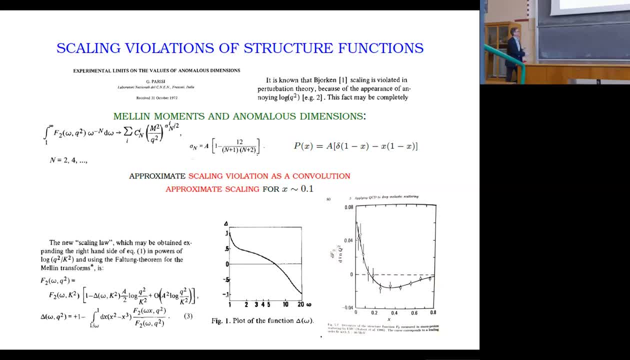 Now it turns out that this idea is almost correct. I mean, what I'm showing here is a plot from Dick Roberts's old textbook from the mid-90s, and it shows this same function now as a function of x, which is the reciprocal of omega. 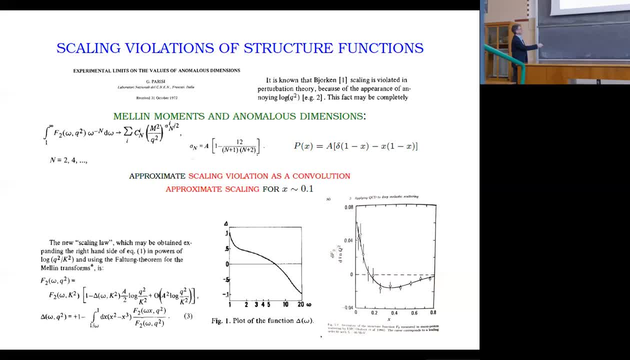 So you see that the qualitative behavior and the change of sign around 0.1 is right. Unfortunately, the slope is wrong in the sense that this goes In the sense that this goes down as omega increases, while this goes down as 1 over. 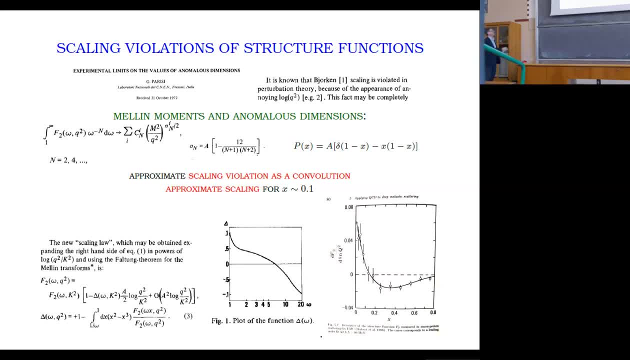 omega increases, But the idea that there is an approximate fixed point in the middle where the data sit is actually essentially correct. The other interesting observation is that this whole line of argument is based on looking at the evolution of moments and then turning that into an equation for the evolution of 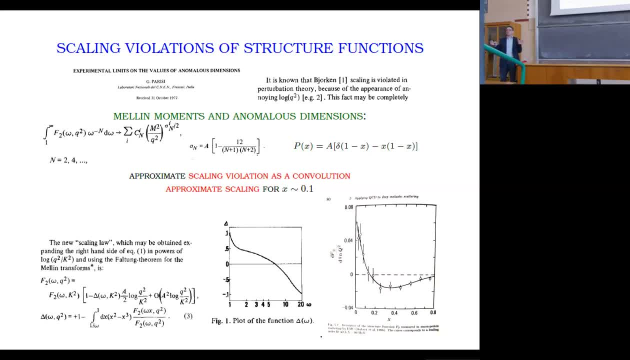 the structure function. Now, this is motivated by the desire of having predictions for something You actually measure, which is the structure function. But what it does is it produces something which starts being very close to the Altarelli-Parisi equation as we know it now, because the product structure of Mellon moments turns into a convolution. 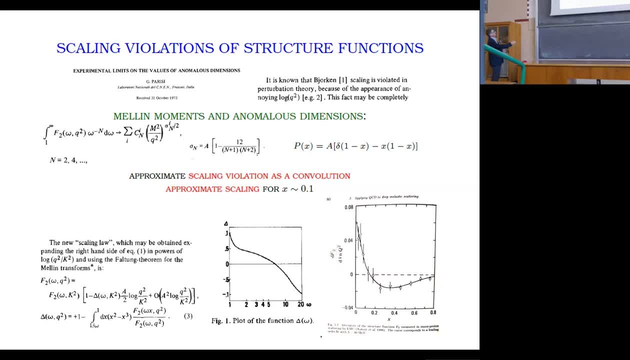 structure using the Fulton theorem, which means convolution theorem, of Mellon moments, of Mellon transform, one finds, So one starts thinking about anomalous dimensions being the Mellon transform, The Mellon transform of something that we would call and was called splitting function, which is then convoluted with the structure function itself. 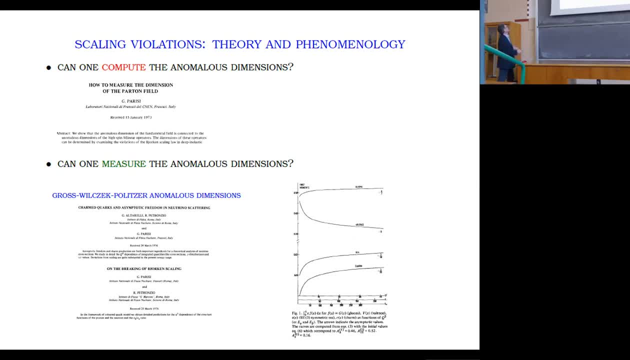 At the same time, Georgian collaborators were asking a number of questions like: can one compute the anomalous dimensions? So at this point the anomalous dimensions had been computed by the American group of Gross Wiltschek Politzer using asymptotic freedom. 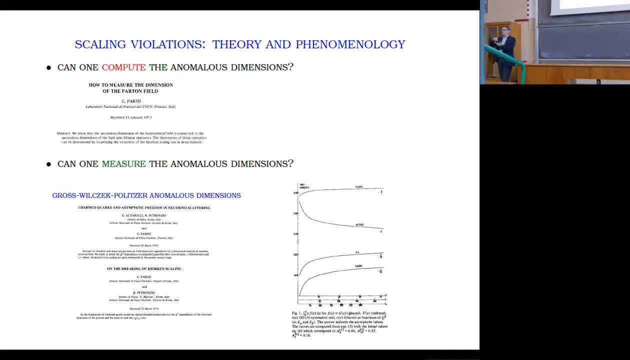 And so there is an attempt to relate the anomalous dimensions to anomalous dimensions of the fundamental underlying fields. And there is also the question: can one actually measure them in experiment? There is this very nice paper, written together with Guido Altarelli and Roberto Petronzio: 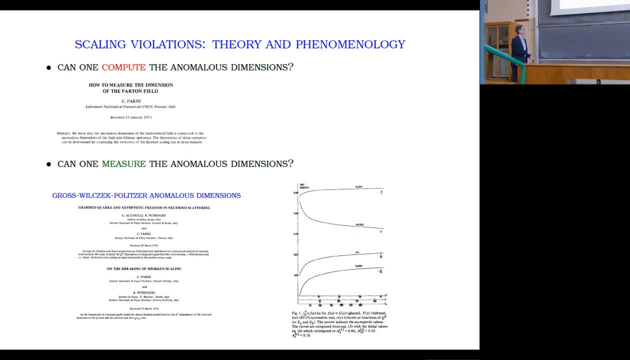 where one finds a plot of the second moment. So these are the momentum fractions carried by valence C gluon. This is a completely modern plot. I mean this you find in present day phenomenology papers, And the idea is that then, by looking at the scale dependence of the momentum fractions, 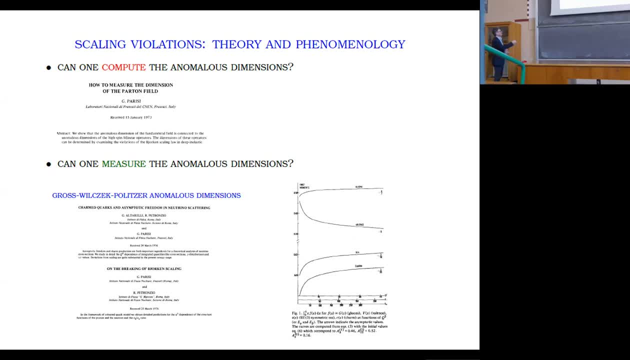 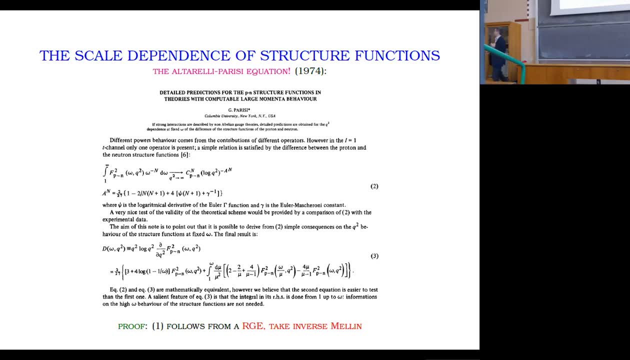 carried by the different kind of constituents. You could actually verify whether the anomalous dimensions are right or wrong. But the paper which I did not well, I vaguely knew about, but I found most striking so that I'm reproducing most of it here, is a paper which Georgia wrote pretty early in 1974,. 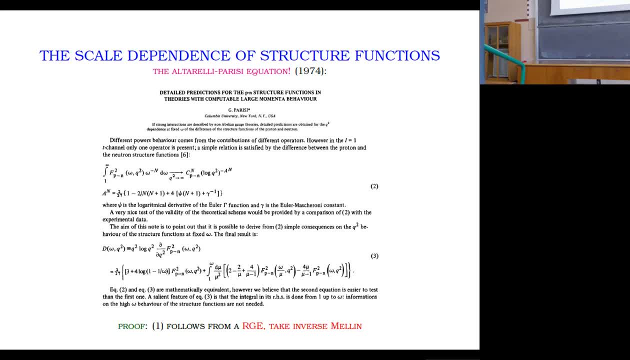 trying again to ask the question: can we phenomenologically see anomalous dimensions in structure functions as we measure them? And the answer Georgia gave was the following. So he starts again by noticing that the moments, the moments of the structure function behave like log Q square raised to a power, and the power is the anomalous dimension. 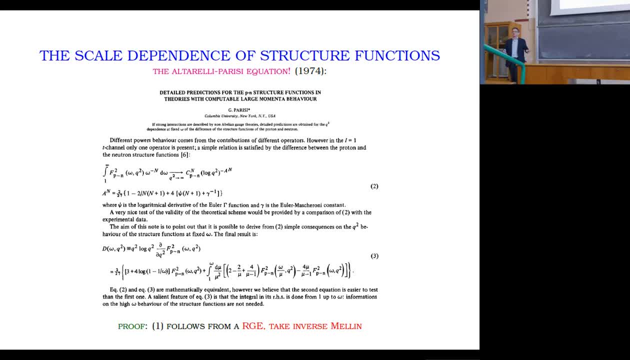 By this time the anomalous dimension had been calculated. So this is no longer a conjecture, but it's the result of the calculations by Gross, Winchek, Pollitzer- the founding fathers of perturbative QCD- And then Georgia makes the following very striking, surprising observation: 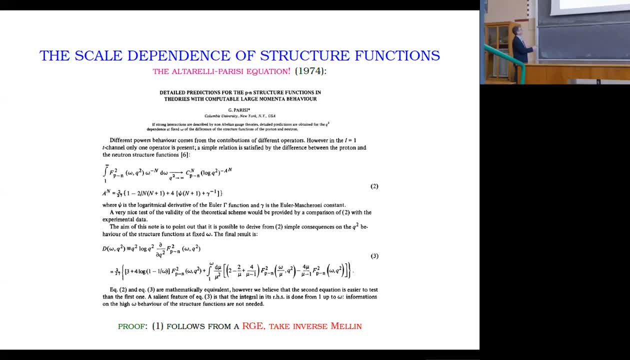 So the aim of this note, it is to point out that it is possible to derive from two- two is just scaling- with anomalous dimension- simple consequences on the Q square behavior of the structure function at fixed omega, And what is written here is basically the Altarelli-Parisi equation which is obtained. 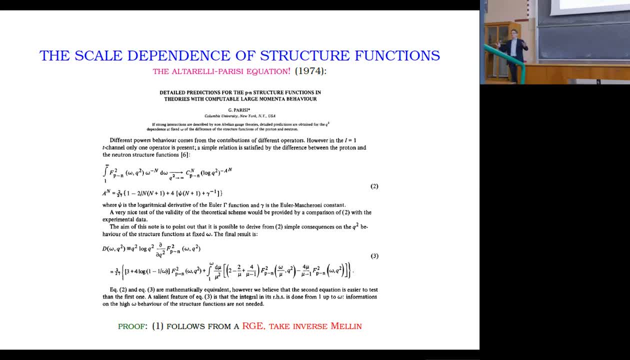 by simply looking at the scale dependence of moments of structure function and then noticing that if you take an inverse Melling transform and you look at this as the solution of the differential equation, then you get an integral differential equation for the structure function which tells you: 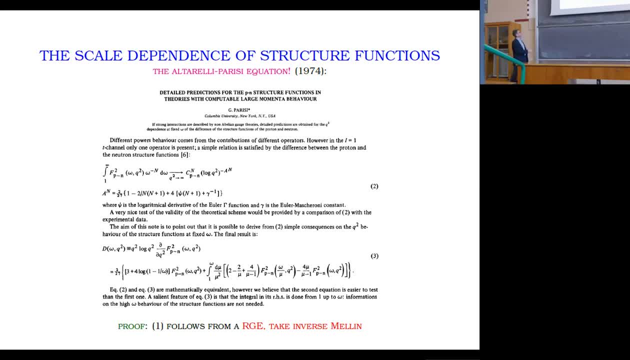 that the scale dependence, the logarithmic scale, depends on the structure function, is given by the convolution of some function, which is the inverse Melling transform of the anomalous dimension, with the structure function itself, which is, of course, the Altarelli-Parisi. 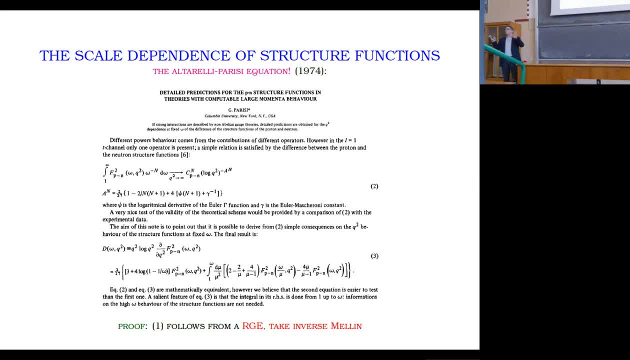 equation which is here found by completely, you know, formal mathematical manipulation. And Another comment that Giorgio makes is: you know, these two formulations, the operator and, and you know, convolution formulation, are mathematically equivalent. 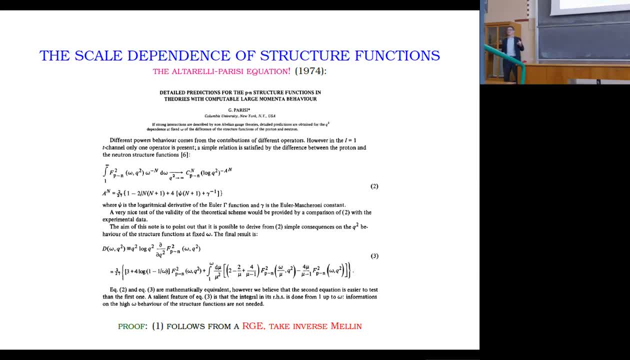 However, we believe that the second equation is easier to test. So you see, it looks like the motivation is is is not not yet trying to understand where it comes from, but rather where you can actually see it in the data, which I found quite interesting. 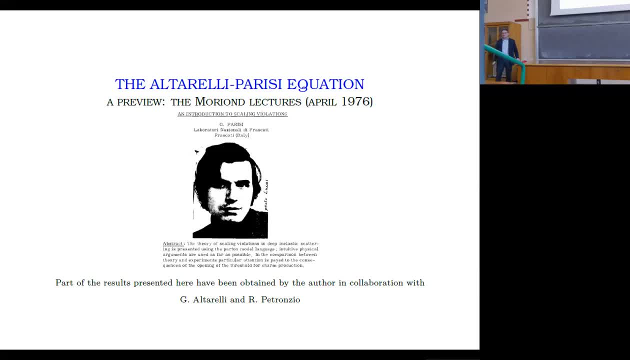 And by the time we get to 1976.. Actually, the Altarelli-Parisi equation as we know it now starts appearing and is first presented in a set of lectures that Giorgio gave at the Morillon conference. You can still find the write up. 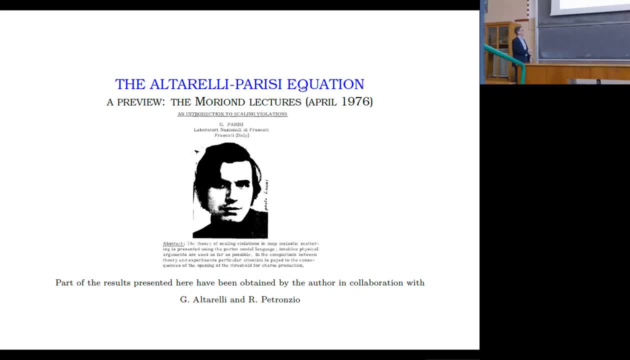 They have a note which says: part of the results presented here have been obtained by the author in collaboration with Vito Altarelli and Roberto Petronzio. And then, as we shall see in the beginning of the Altarelli-Parisi paper, there is the 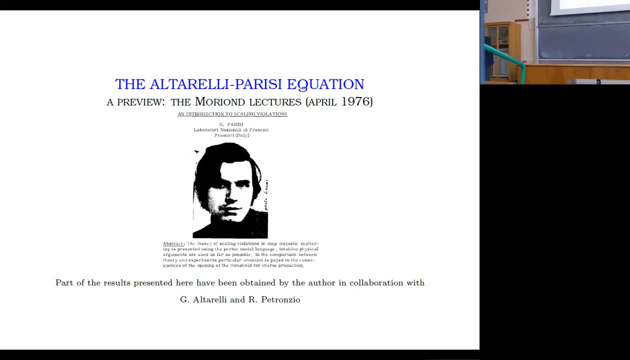 reciprocal sentence. Some of the results presented here were already published in, and you know. this is shown And you can see the abstract, which starts being very close to what we know as the major Altarelli-Parisi breakthrough, Namely the theory of scaling violation in deep magnetic scattering is presented using 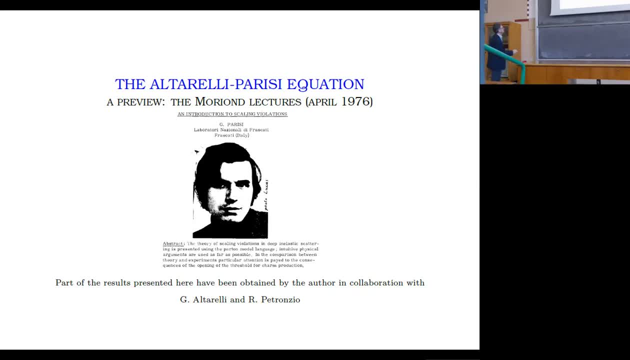 the part on model language, you know, asymptotic freedom, in part on language, Intuitive physical arguments are used as far as possible, And then in the comparison between theory and experiment, particular attention is paid to the consequence of open logic. So again, it is remarkable that there is this guiding principle of trying to actually 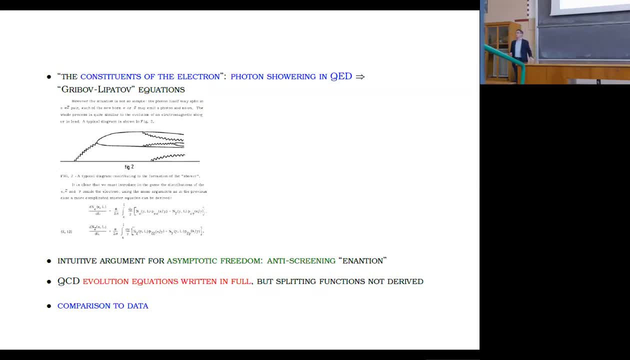 see things in the data. Now I'll just spend a few minutes about this preview of the actual Altarelli-Parisi paper and then move to that, But I cannot resist the temptation of showing you a couple of gems that are to be found. 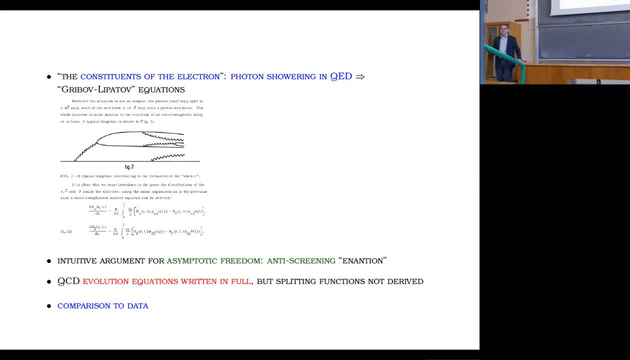 in this paper, So the first part of this set of lectures. It's actually doing QED rather than QCD And what it does is it describes what we would modernly call part on showering, or rather photon showers, in QED. 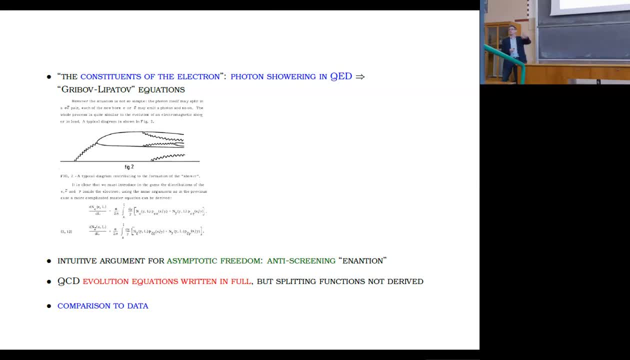 So there is a chapter which is entitled The Constituents of the Electron, where the line of argument is: an electron can radiate a photon, and then a photon can radiate an E plus, E minus pair, and then the E plus and E minus in turn radiate photons. 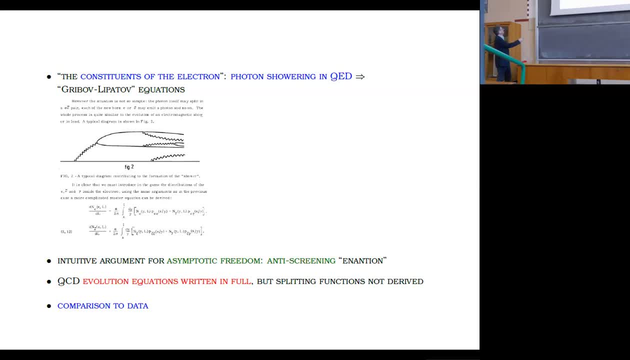 And then you get the showering process, Which can be described by two equations, which are the Altarelli-Parisi equations, except for QED. they are modernly known as the Griebov-Lipato equation, because they had been developed. 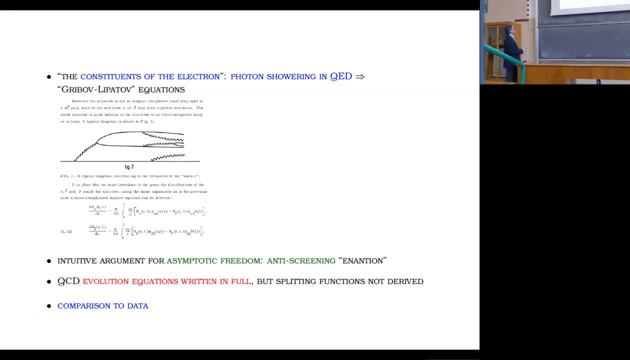 by the Russians, completely independently, I guess. And then, well, so there is this nice lengthy discussion of QED before moving to QCD. This is followed by an interesting chapter which reproduces: Okay, So this is a description or a physical picture of asymptotic freedom that is now to be found. 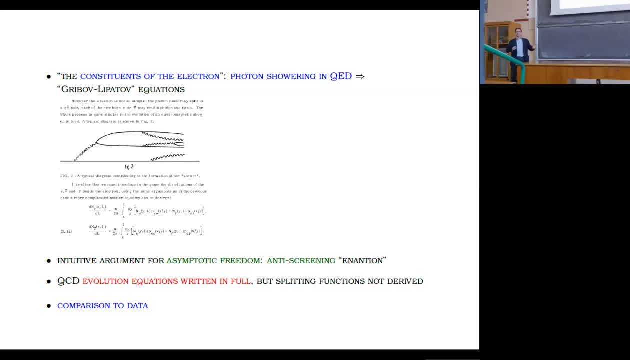 in any textbook. I mean, you open Peskin and you find it. So the idea is, you first start with QED and you observe that in QED if a photon splits into an E plus, E minus pair, then the vacuum can behave as a dielectric because the E plus 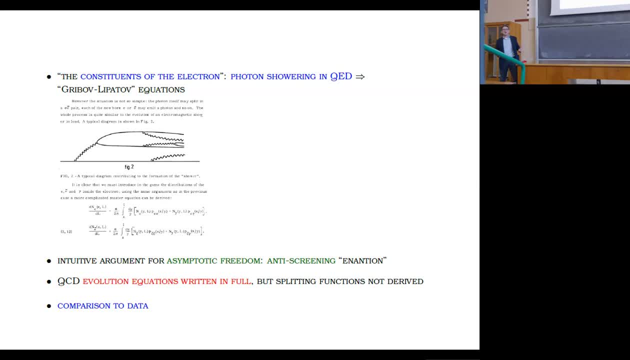 E minus pair aligns with the field and therefore it screens the charge. So when you go afar, you actually see as long distances You actually see, Okay Okay. So you see a smaller charge. and when you get closer, so at high energy in QED, you see. 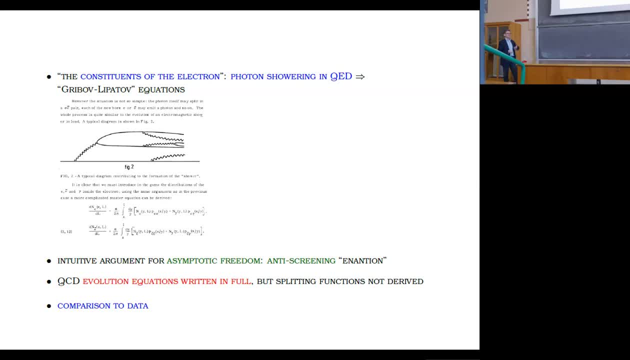 a bigger charge. but then Giorgio says something strange can happen which is the opposite, So you can have something which is called the enantion. You know, I didn't go to a classical high school so I didn't study Greek, but I guess. 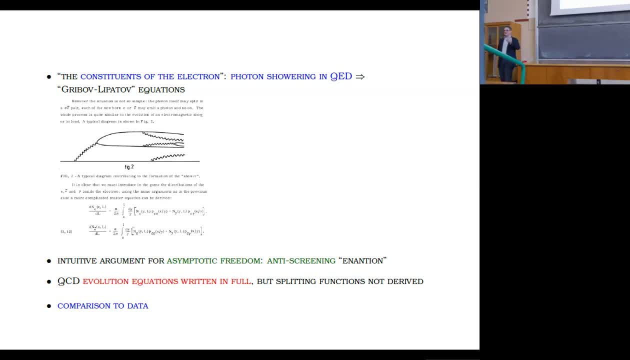 this means something which behaves in the opposite way, which means that the vacuum anti-screens- which, of course, is what we know now- happens because of gluons, and then you get the anti-screening picture. Okay, So this is asymptotic freedom, because when you get closer to the charge, instead of it. 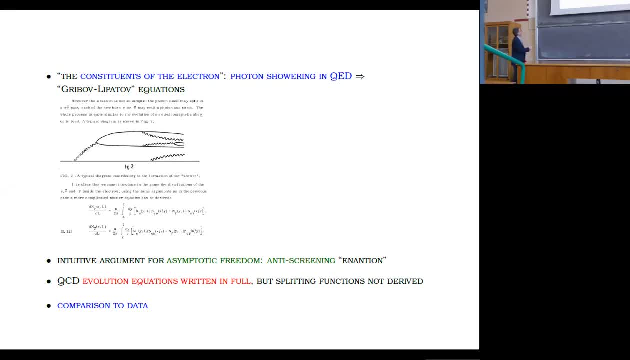 being larger, it's actually smaller, which is asymptotic, free, Okay. And then, after this nice physical picture is given, the QCD Altarelli-Parisi equations are written down in full, but there is no derivation of the splitting function. 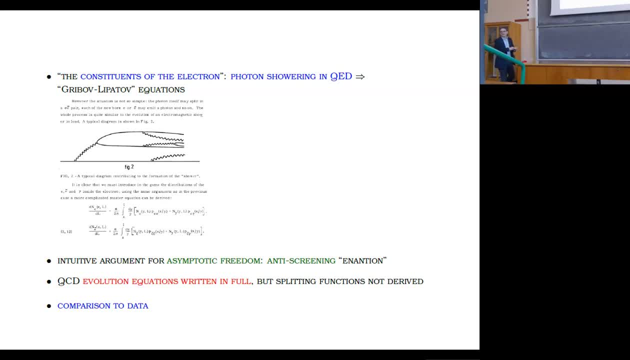 There is no calculation of the splitting function, So this is the only thing that is missing in comparison to the subsequent paper. And then there is a very detailed comparison to data, including an extensive discussion of charm, which at the time was A novelty because we were talking about 1976 and the, you know, the JSI revolution from. 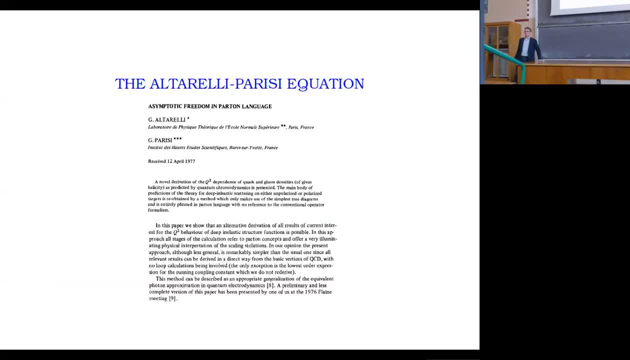 was from a couple years earlier, And this brings me to the paper that gives the title to this talk. I'm reproducing here the whole front page because, you know, I think it's worth taking a look at the paper, and then I would spend some time walking you through the actual calculation. 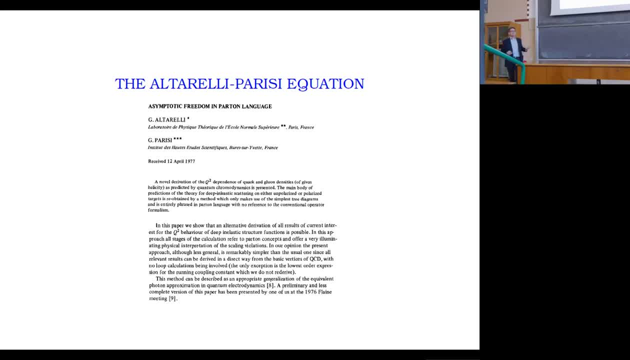 in the paper. Of course, it's a textbook calculation these days, but this is one of these papers where the original presentation Is. you know, sometimes when you look at old papers, you look at them and they are impossible to understand. 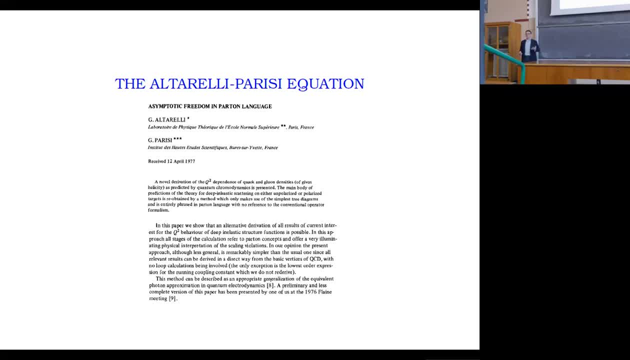 But there are rare cases in which, instead, you look at your original paper and the presentation is so nice and clear that all subsequent textbooks basically reproduce it, with maybe some small variation. So you know, the rest of the calculation is essentially identical up to some small detail. 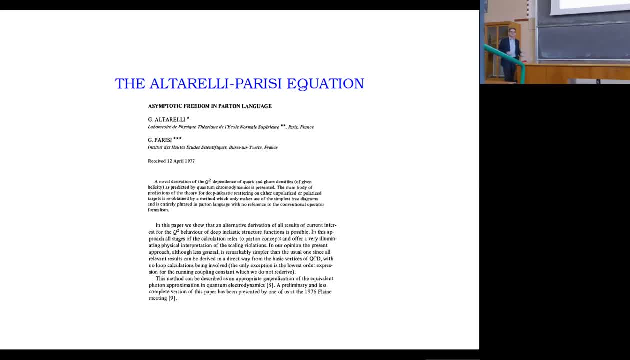 that I will comment upon, to what you find again in Peskin's textbook or in any textbook, but it's still worth having a look. But before doing that, Okay, I'd like to briefly call your attention on both the abstract and starting sentence, because 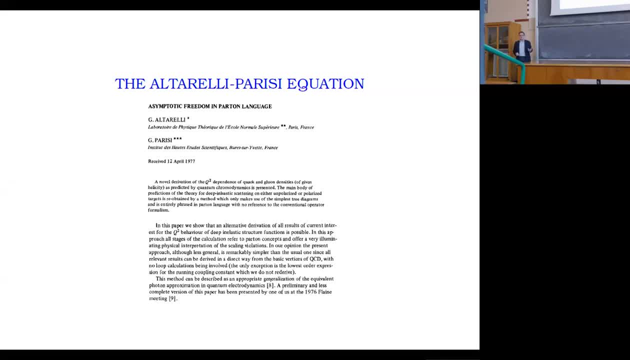 that allows one to appreciate what this paper is really about. So you know, the abstract is similar to that of the Morion proceeding. So a novel derivation of the Q-squared dependence of quark and glue on densities. So now it's quark and glue on densities and not structure functions predicted by quantum. 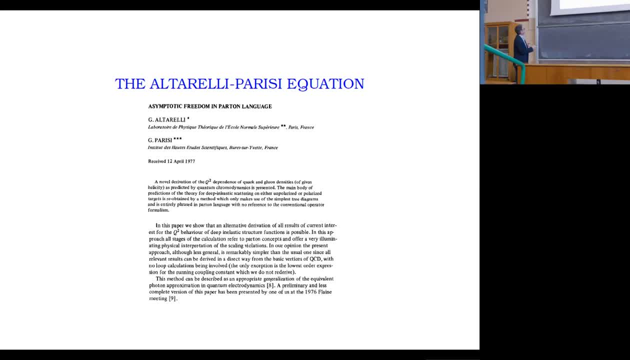 chromodynamics presented the main body of predictions for deep gymnastics, scattering, polarized or unpolarized, Can be reobtained by a method which only makes use of the simplest tree diagrams and it's entirely phrased in part on language. 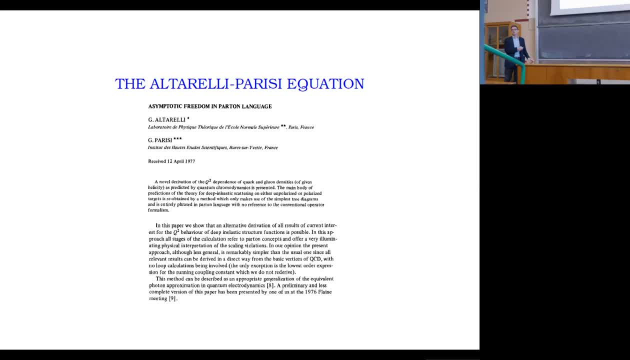 And then you know, the first sentence says this in an alternative derivation of modern being, gross, wheelchick and so on, results on the Q-squared behavior of DIS. And in this approach all stages of the calculation refer to part and concept. 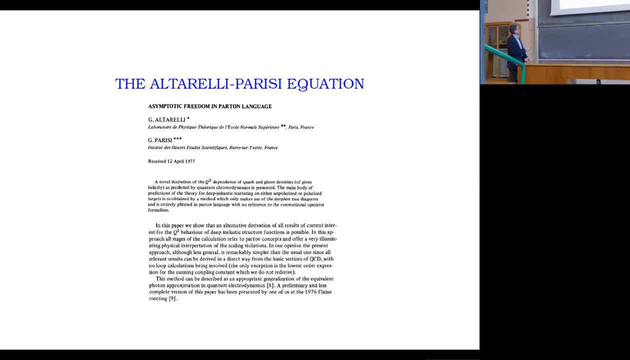 This is the title of the paper after all, asymptotic freedom, in part on language, and in our opinion, the present approach- Although that's general- is remarkably simpler because results can be derived in a direct way from the basic vertices of QCD, with no loop calculation being involved. 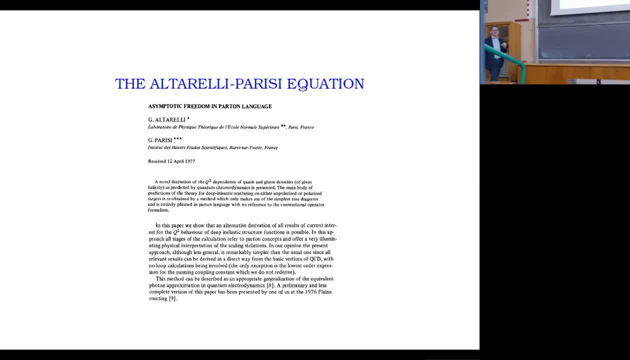 So you see, what this paper is really about is understanding the underlying physics of scaling violations as found using the Wilson expansion, which is something that sometimes people don't appreciate. I mean, I've seen sometimes, you know, people saying, well, this should be called the D-GLAB. 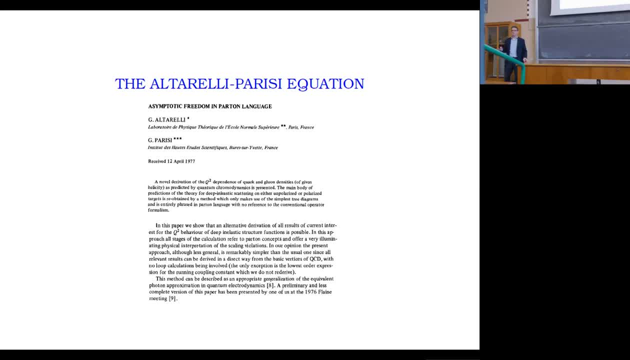 equation because it was written by Doxitz and Leibov-Ripatov in previous paper. Of course you know you can call things any way you want, but you know a friend of mine used to say that calling this the D-GLAB equation is like asking whether the Vikings 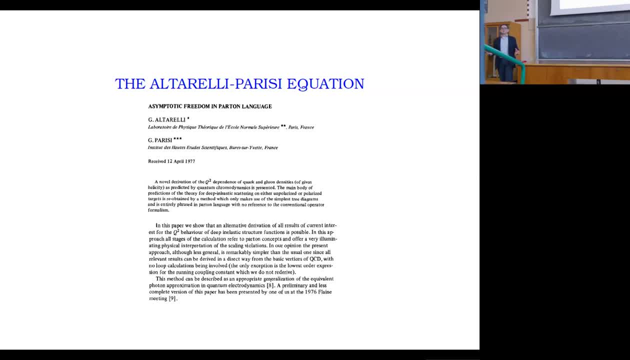 discovered America, which means the following: that you know, when we say discover America, we don't mean that someone went to America and set foot there. We mean that someone understood that you know the earth is round and you could get to some continent which is on the other side of the ocean. 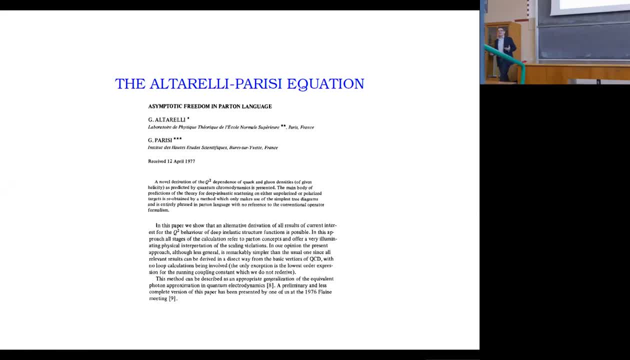 And then come back and you know understanding what that means. it's not just putting the foot there. So you know, discovering something does not mean just writing the equation, but understanding what it means. Yes, May I add that this is another Georgiou paper, because Georgiou always says that the important 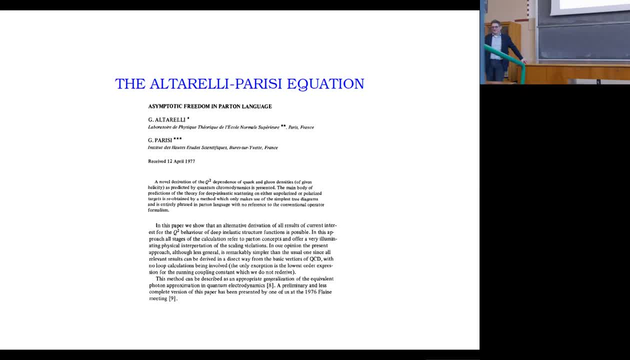 thing is not discovering something first, but discovering it last. Okay, I didn't know that, but yeah, Okay, No. So Georgiou always says that what is important is not discovering something first, but discovering something last. And this is exactly what you say. 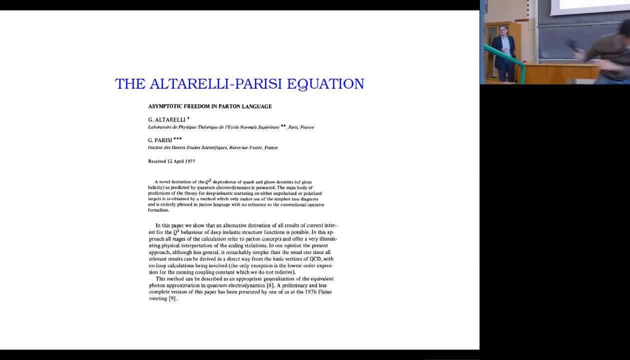 Right, And he says about America, Okay, Yeah, Well, this was a fellow graduate student of mine that used to say that when we were studying this for our general examination at MIT, and you know, and you know, come on, I mean. 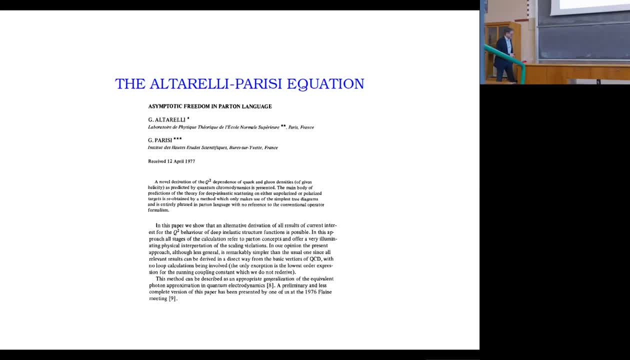 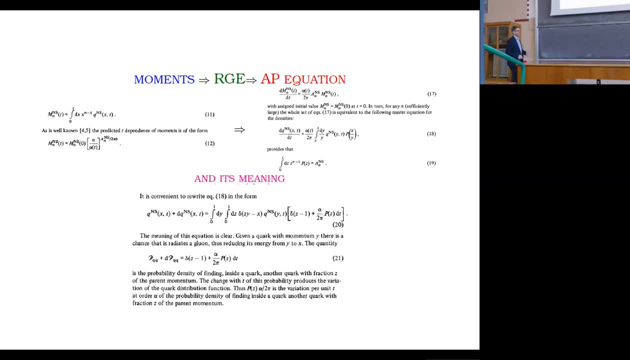 he had this quote and then he left for Wall Street. Okay, So let me now get through. I mean walking through the Al-Fareli-Parisi Derivation, because it's- you know, it's such a classic that it's worth going through. 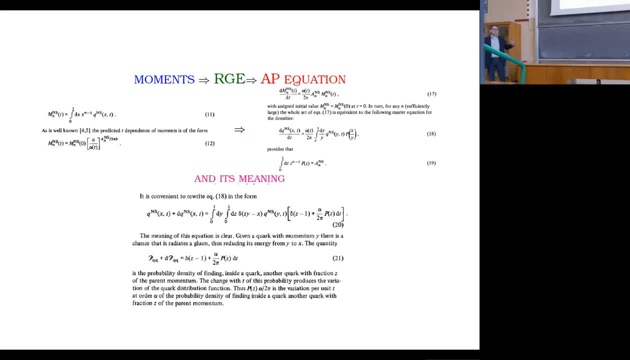 Once again. you know it's like when you hear a Beethoven symphony that you've heard so many times, but it's still very nice to hear it because you know of the sheer beauty of the art. So the argument starts like the anticipations that I've been talking about 15 minutes ago. 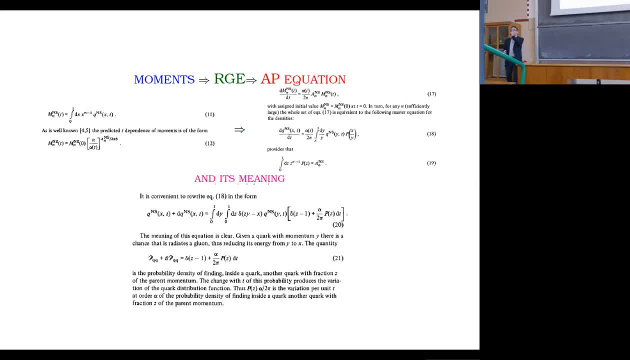 So first one takes moments, except that now it's no longer moments of the structure function, is really moments of the quark distribution. So you have a quark distribution, no longer the structure function. And then you say: as well known, the predicted. 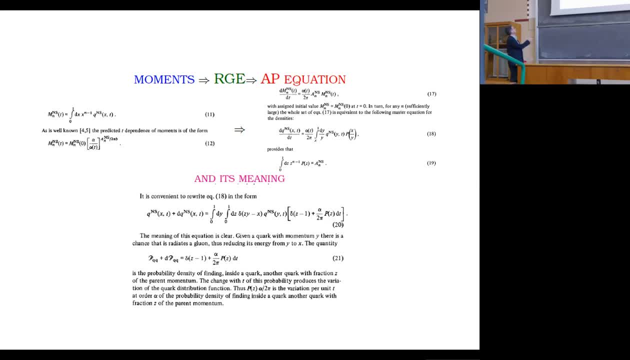 T is log Q square. the predicted logarithmic dependence of the moments is of the form And interestingly, the log Q square is not written as log Q square but it's written as a strong coupling as alpha S. Of course alpha S goes like one over log Q square. 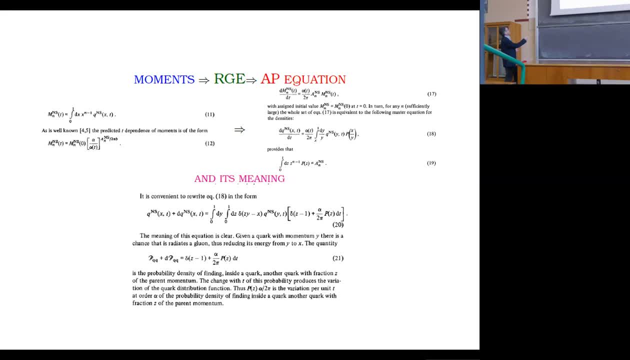 So it's like log square raised to a power of the anomalous dimension by well, divided by the first coefficient of beta function, because you have the alpha S and not log Q square. And then the observation is: well, This equation, The equation here for the Q square, dependence of moments, can be viewed as a solution of. 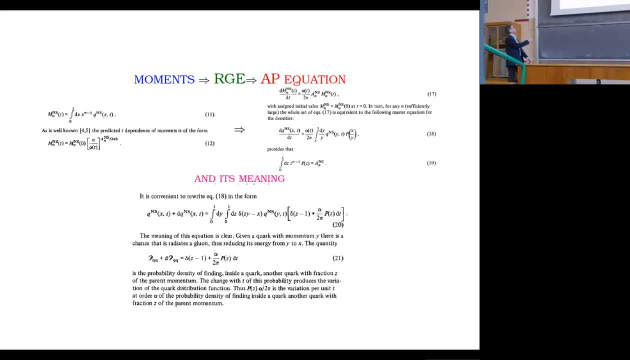 a simple first order differential equation for log Q square with the anomalous dimension, which is kind of trivial, And then, by taking the inverse Mellon transform, which was the insight which previously was given as a purely mathematical curiosity, you can rewrite this as the log derivative. 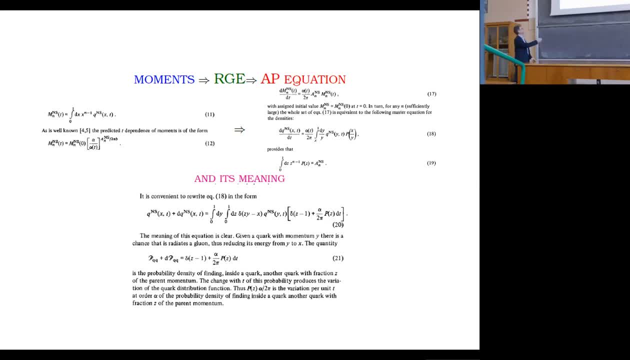 of the part and distribution itself, No longer it's moments. You take the inverse Mellon transform, which is then the convolution of some function, P, with the part of distribution itself, where P is the function whose moments, the splitting functions, whose moments are the anomalous dimension. 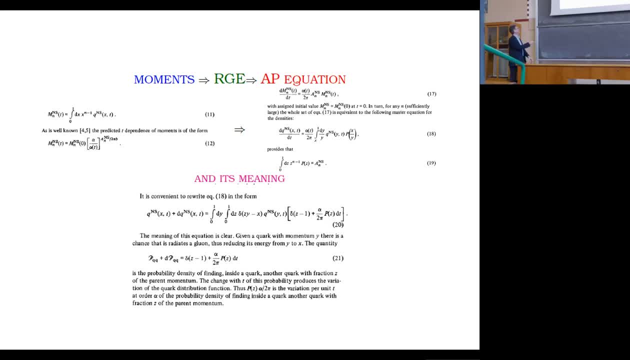 And then you know: stop. What are we saying here? Then there is a comment. Well, we can rewrite it in the form, And then the meaning of the equation is clear: Given a quark with momentum Y, there's a chance that it radiates a gluon, thus reducing its. 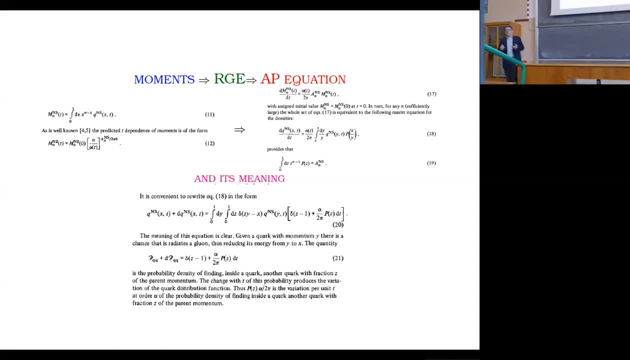 energy from Y to X, And then you define a differential probability of splitting, and then you understand That this, which looked like a mathematical curiosity, is the inverse Mellon transform of an equation whose solution is something we knew- actually has a direct, simple, physical. 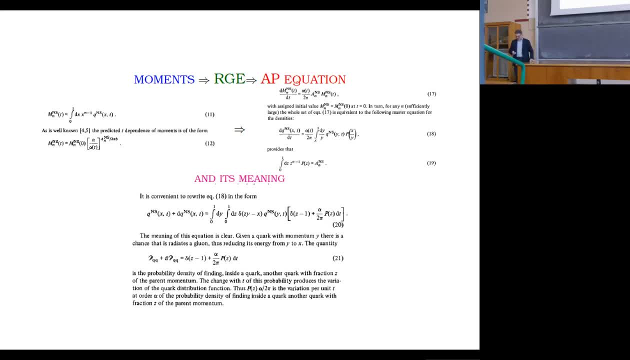 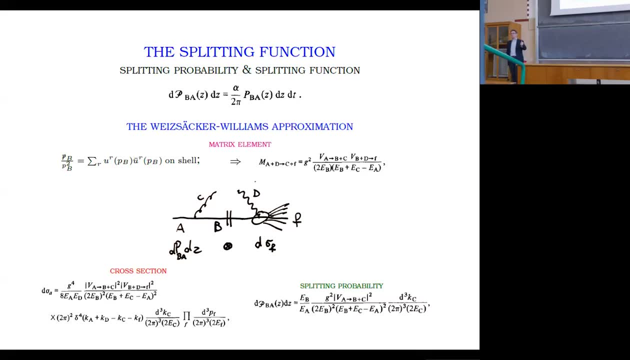 interpretation. It describes the part and branching process which I had in the previous slide in QED. OK, So at this point the new part of the paper which was not in the Morion lectures comes with a direct calculation of the splitting function from Feynman diagram. 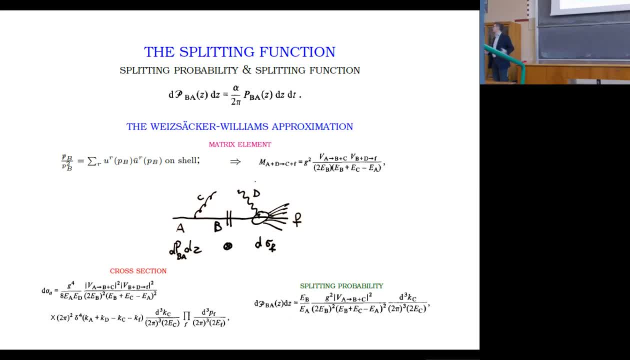 And this turns out to be remarkable, remarkably simple as the absolute, Because the paper said: I mean something which you can do by not calculating any loops, just calculating three diagrams. So it is done in various steps that I'm going to walk you through. 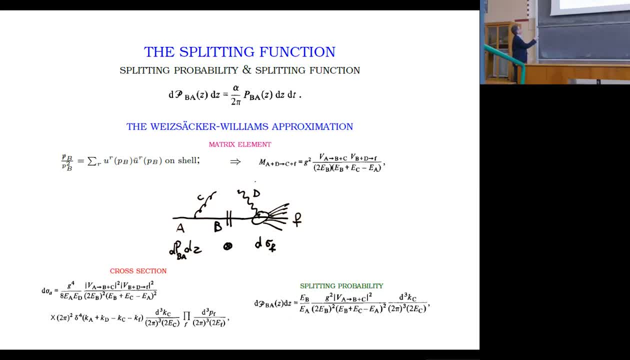 So of course the first step is relating the splitting probability to some splitting function by pulling out a differential factor of T. T is log Q squared. So you write this as a differential in log Q squared And then you calculate the process of radiation. 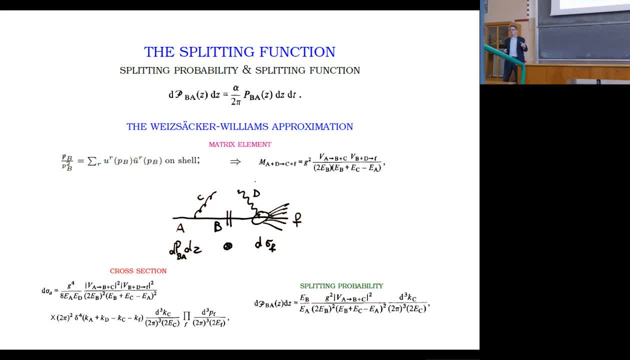 OK, Using the Weitz-Secker-Williams approximation which, as we saw, appeared in a very old, well very old- in a much older previous QED paper of Giorgio, where it was used as a device to calculate E plus E minus into E plus E minus gamma. 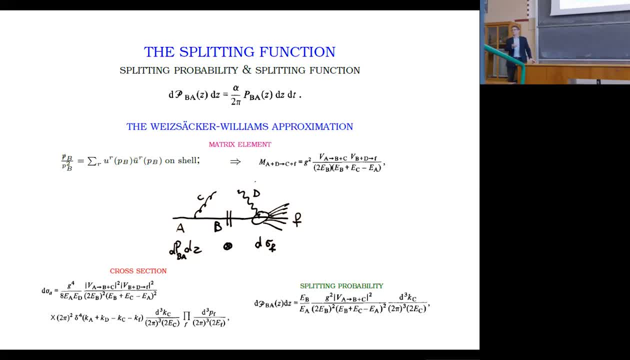 So the idea here is the following- I'm drawing it here. This is something which we've seen many times and taught the students. You have deep, elastic, scattering, a virtual photon hitting a quark and producing a generic final state F. Now the quark, before being hit by the virtual photon, radiates a gluon and then you realize: 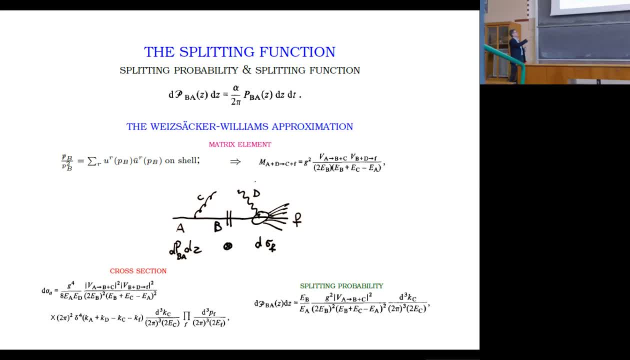 that, in the region in which the radiated gluon is almost collinear, is almost parallel to the incoming and outgoing quark. you can treat the intermediate state as a quasi-real state. You can put it almost on shell, which means that you can- well you know- a fermion propagator. 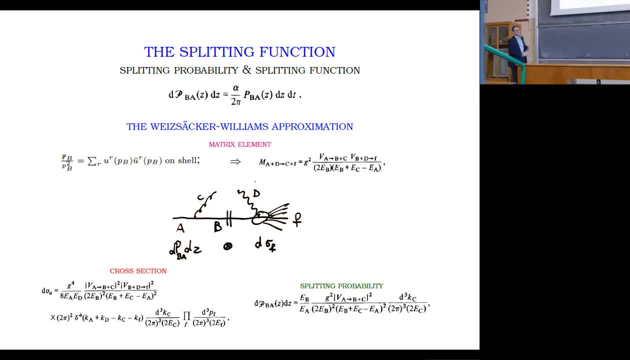 that appears here. That's divided by P square. You can write it as a sum over on shell intermediate state, and then the process splits in half, which is the standard derivation that you find it in Peskin or in any other textbook, which means that the matrix element can be written as the product of the matrix element. 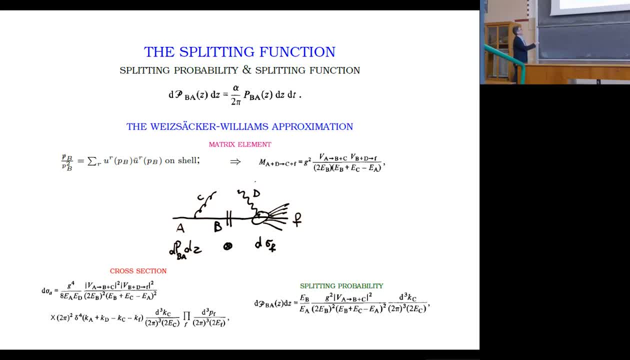 of the quark splitting into a quark plus a gluon times the matrix element of the quark absorbing the photon and producing the final state. And, of course, the power of the argument is that the radiation process is completely decoupled from the final process which is happening. 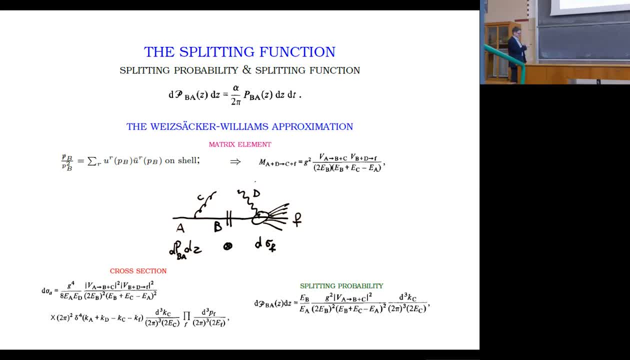 Later. there is a technical detail here which is peculiar and which I'm going to comment upon in a few minutes, But let me first note that then. what this means is that if you calculate the cross section for the whole process- because the matrix elements split like this- you can write the: 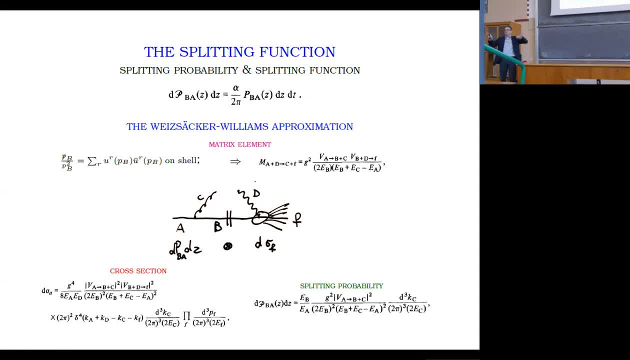 cross section as the product of two sub cross sections. So the process really splits into a splitting probability times the final process And therefore the splitting probability is given by a universal expression which only depends on this splitting diagram here and which does not depend on the particular physical. 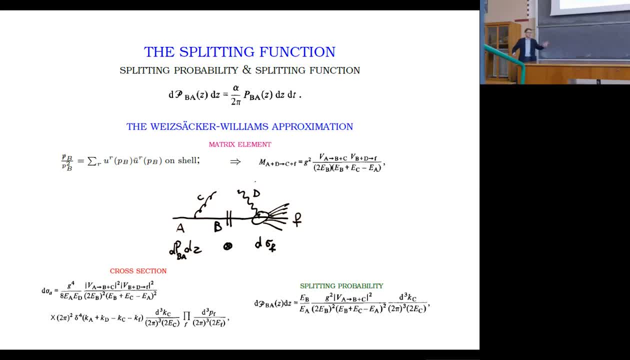 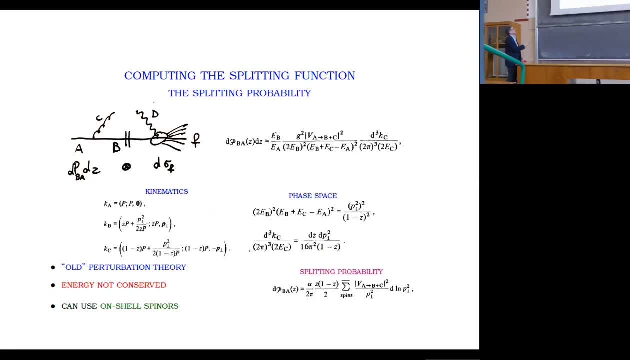 process, be it deep magnetic scattering, Drell-Yann, Higgs, whatever you know, part and branching is universal and process independent. The next step is then calculating the splitting probability, so calculating the splitting function, And this is done. this means you know calculating this expression here. 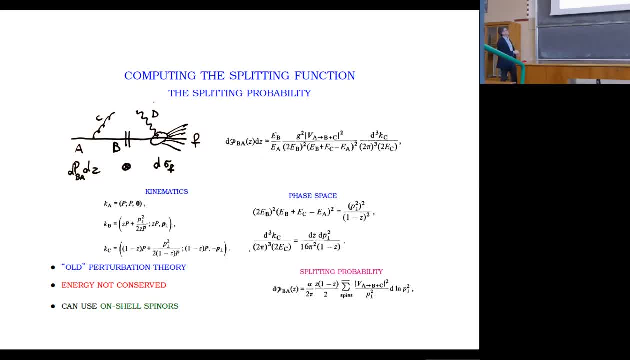 So, if you wish the a, c, b part of the diagram which I'm drawing here Now, this is done. now, this is the peculiar aspect of the calculation. This is done by using so-called old perturbation theory. Old perturbation theory means that you write the momenta for a, b and c in such a way: 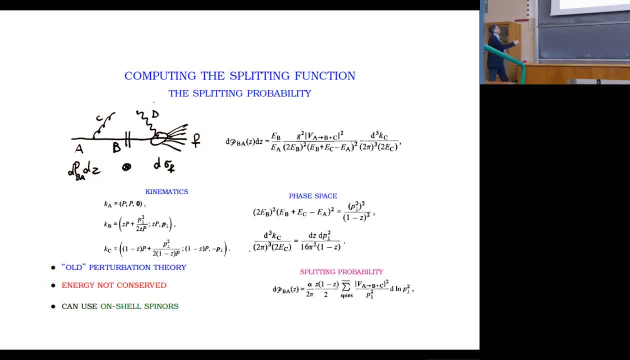 that all three of them are on shell, at least to first order, in transverse momentum square, because we are looking at the small transverse momentum where you have the collinear singularity but energy is not conserved And indeed you may have noticed that the perturbation expansion formula has an energy. 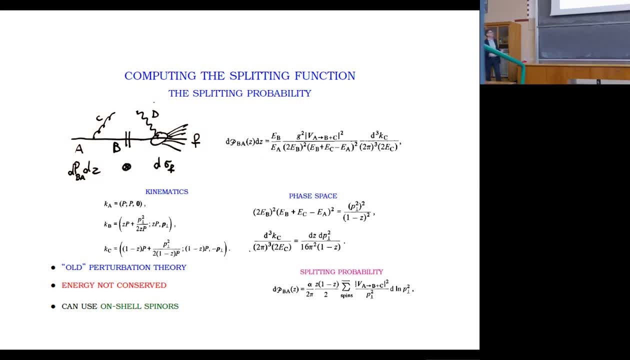 denominator, which would be zero. So you know it would explode if energy was conserved. Now using old perturbation theory, you know the paper says is not necessary, but it's actually an extremely clever trick because the calculation then becomes much simpler. 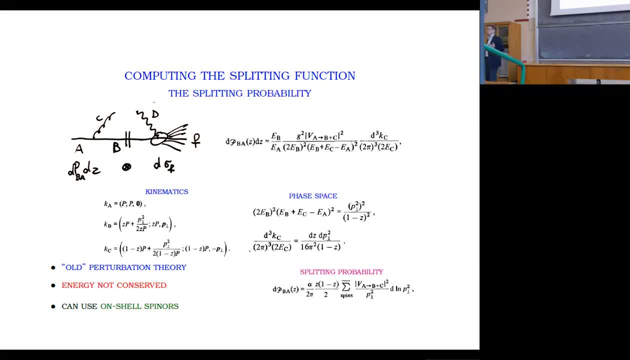 So if you compare this again to the calculation you find in textbooks like Peskin, it's actually much easier because thanks to the use of old perturbation theory, the calculation becomes much simpler. So you have to pay the price of not conserving energy, but what you gain is that you have 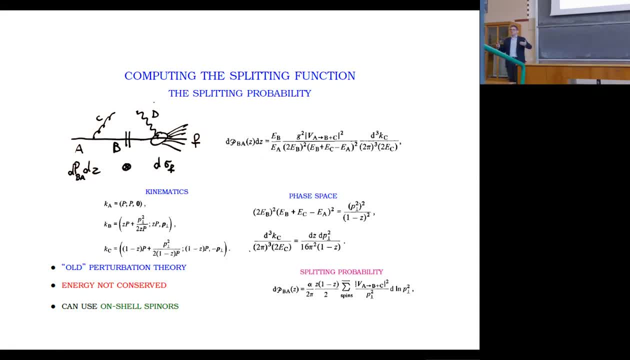 an on-shell intermediate state and then you can use on-shell spinners so that the calculation of the Feynman diagram reduces to calculating traces in the way we know when you take the square modulus of something with external on-shell spinners. In other words, you're putting on-shell the intermediate state here, while if you do it, 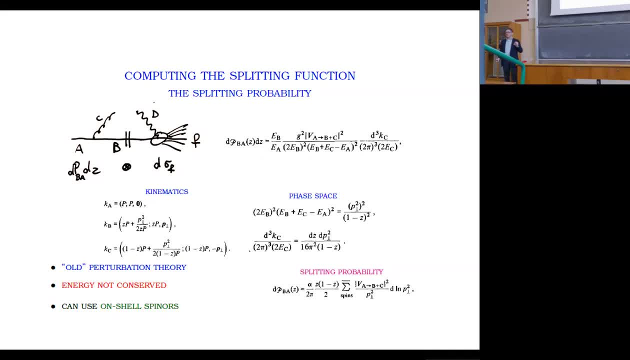 like in Peskin. here you have to have a slightly off-shell state. You conserve energy, But you have a much more complicated expression for the spinner. You cannot do the calculation using traces. You have to substitute the explicit expression for the direct spinner. 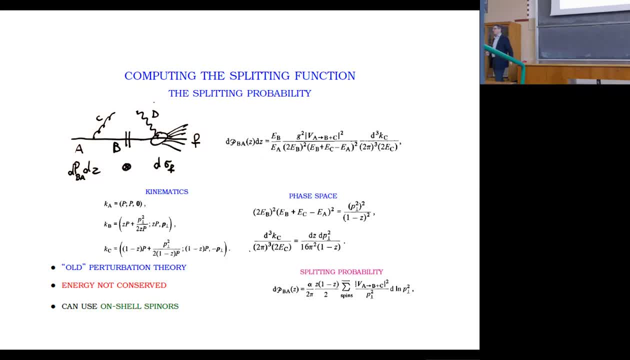 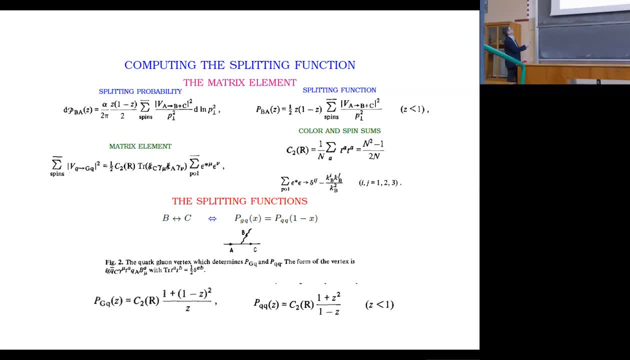 So this is a kind of you know, technical virtuosity which makes the whole thing much simpler. And then, you know, then computing the splitting function is very simple, because you just express the splitting probability. So you know, let me go back. 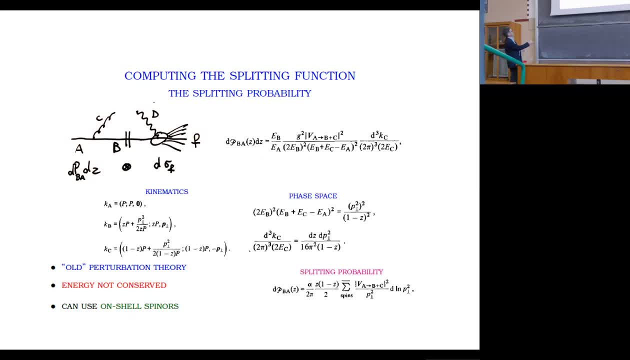 You first calculate the phase space with this triangle. You calculate the phase space with this triangle. You calculate the phase space with this triangle. You calculate the phase space with this triangle And then you find the choice of kinematics. Then you replace the phase space in the expression of the splitting probability. 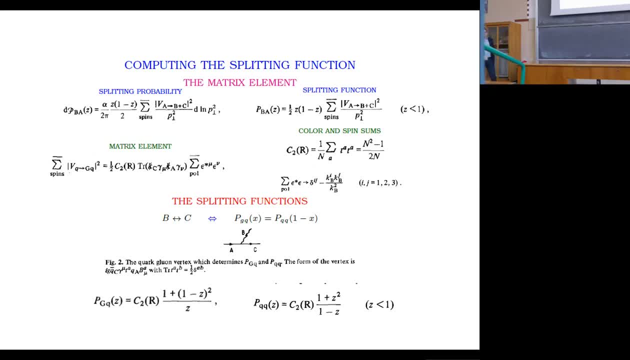 And the splitting function is then reduces to computing a trace. It's reduced to computing a trace because, as I said, you have external on-shell spinners. So then the square modulus is the usual trace, like we teach students when we teach them the first computation of QED. 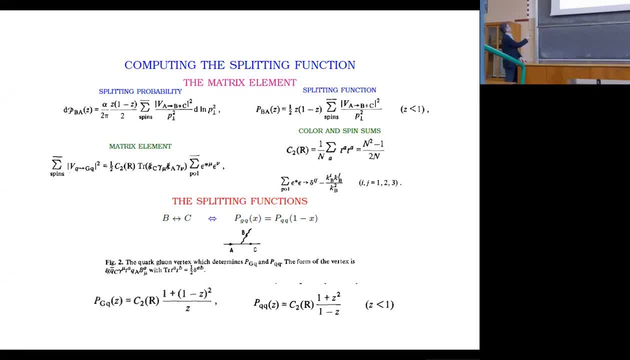 It's a completely trivial straight forward trace with just four Dirac matrices contracted with a photon polarity- Yeah, polarizations- and with the color factor. color and spin sums are very simple and you end up getting the expression for the splitting function. here I'm showing. 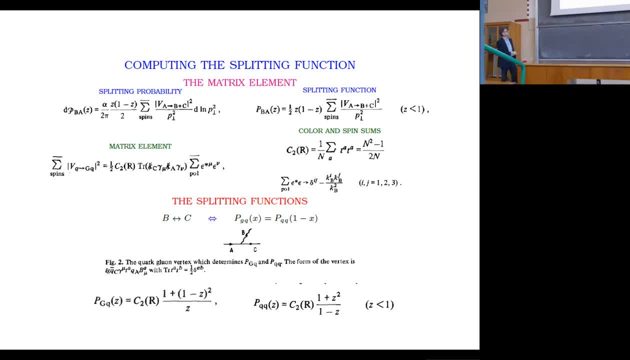 the expression for pgq, so a gluon, so finding a gluon inside the quark. of course pqq, which is finding a quark inside the quark, is the same thing. interchanging x into one minus x, which means interchanging b and c, so with one. 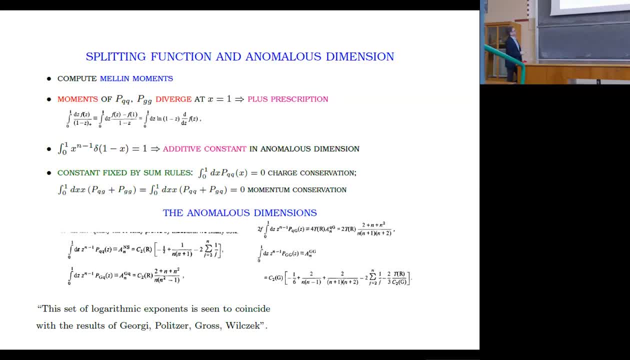 calculation, you actually get two splitting functions. and then there is the question: how does this relate to the operator formulas? well, we take moments, because moments of the splitting function are anomalous dimensions. except that if you take moments, you realize that pqq and pqg actually diverge. the 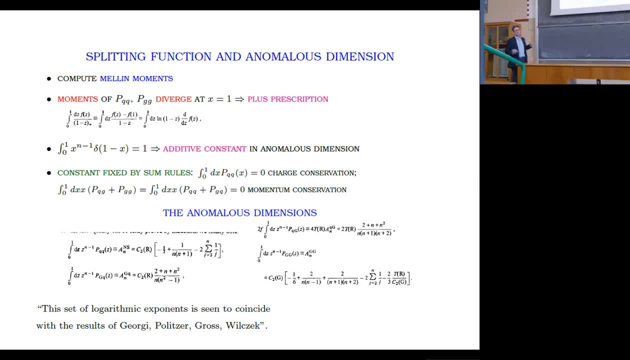 moments diverge. but then there is the observation: yeah, they diverge because we missed a contribution which comes from loop corrections. except that one does not have to compute it, one just replaces the divergent denominator with what we all now call a plus prescription. so you subtract an endpoint term which would be: 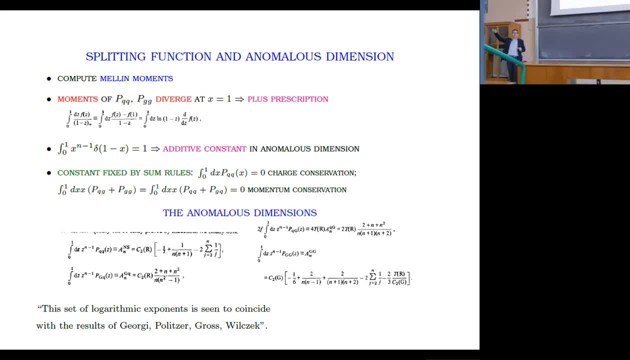 the loop correction, the virtual correction which is proportional to a delta, because the loop correction has the same kinematics as the leading order, the previous order, and then you fix the coefficient of the delta by imposing charge conservation or momentum conservation, which then allows you to determine the constant with the. 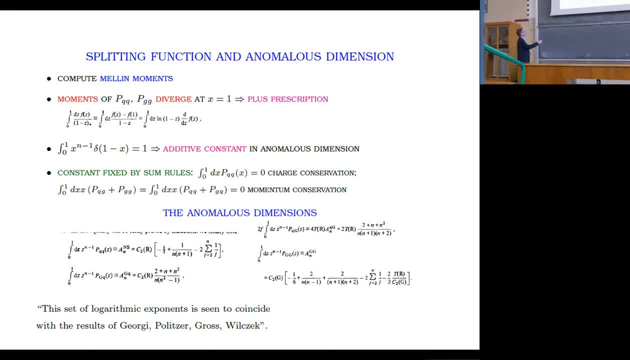 Lagrangian��는, without calculating anything, and off you go and you get the full set of four anomalous dimensions. and then the final comment is: this set of logarithmic exponents is seen to coincide with the results of George I-Politzer-Growson-Wilczik. 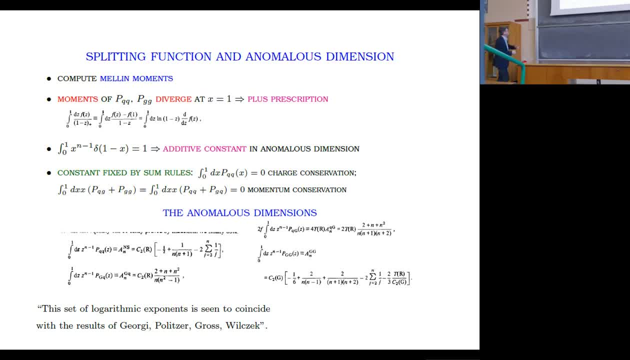 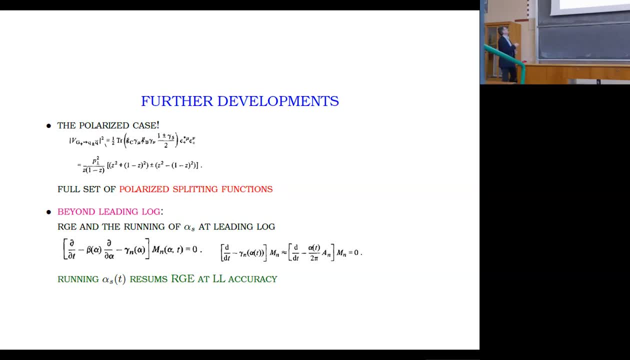 which is almost the end of the paper. it's not the end of the paper because the paper keeps following the argument forward, first of all by redoing the whole calculation in the polarized case. so polarized splitting functions are not something that was the problem of the 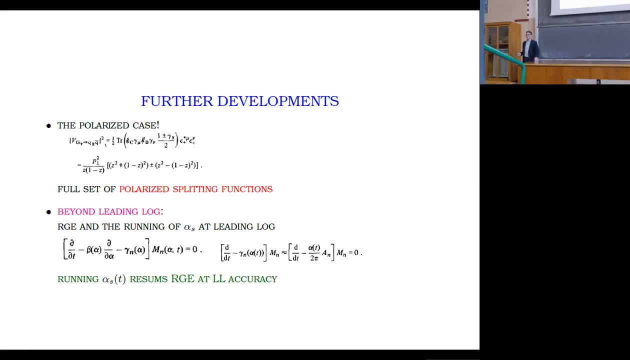 was measured and discussed until the mid nineties, I would say. but they are fully done here. And because of the way the calculation has been set up, it's actually quite easy. You just stick in polarization projectors, so gamma fives, into the intermediate stages calculation. 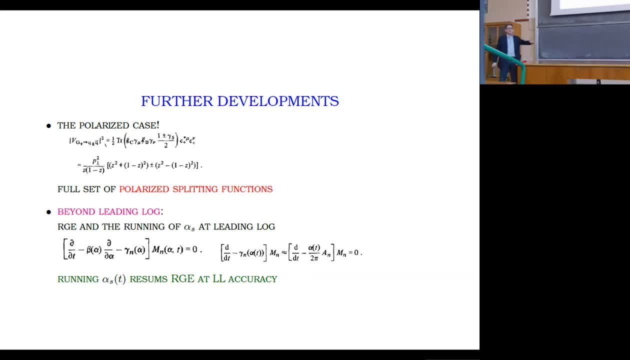 then you get the polarized results And then, finally, there's a question: can we do this beyond the leading order, which is really leading log? because you're summing the leading loss will order And the observation is: well, this argument was so simple. 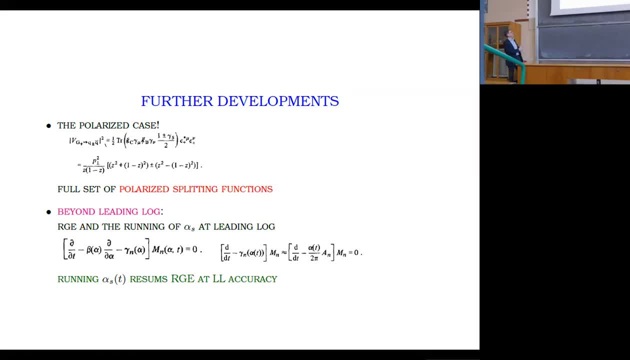 because at leading order the Kalan-Szymanski equation can be reduced to a linear differential equation by simply replacing alpha with alpha S of Q square. But if you go to next to leading order then you have to keep track of the mixing of the logs. 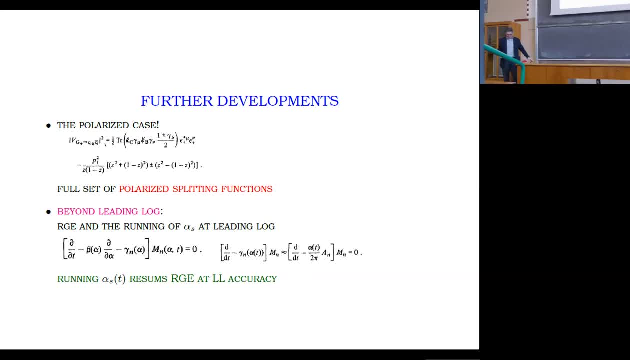 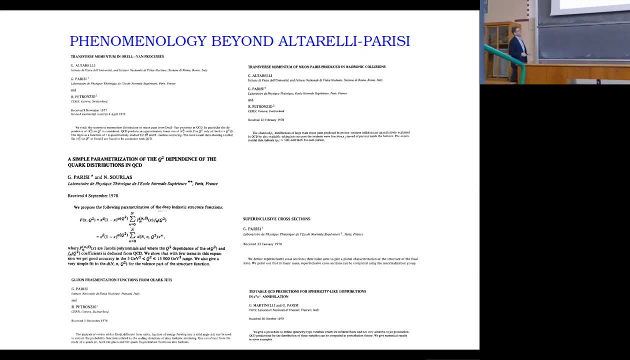 of the running with the logs of the evolution, And this was only done by Kurchi, Formanski and Petronzio a few years later. but you know, this kind of sets the stage for this After this paper- and I'm coming to the end of my talk- 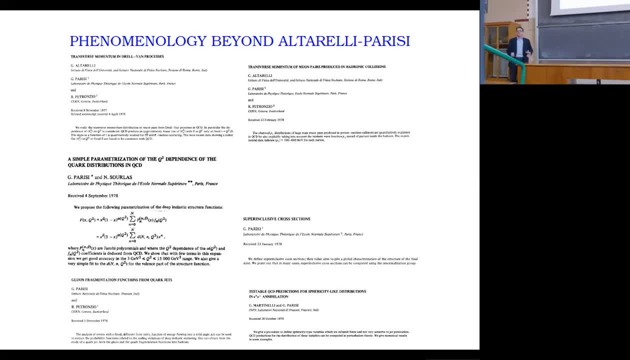 Giorgio actually published a number of FINO papers where you know, having set up the correct formula is now at this point perturbative. QCD is all there, factorization all you want. So one can do trans-repermental in Drellian. 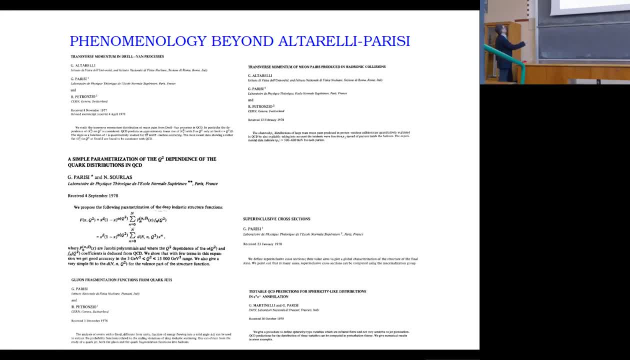 trans-repermental muon pairs produced in Drellian. You know I don't have the time to go through the abstracts- The FINO developments, like parametrizing the Q square dependence of quark distributions, because at this point you have the equation. 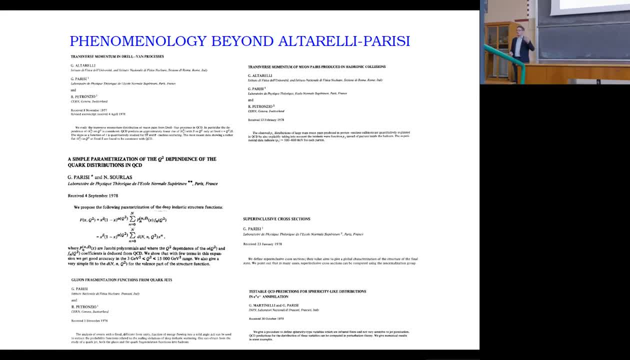 you have the solution, but you can do something which is close to modern part and fitting, except that the functional forms were simpler because at the time the data were not so precise. Then, jet physics, there are, you know, super inclusive cross sections. 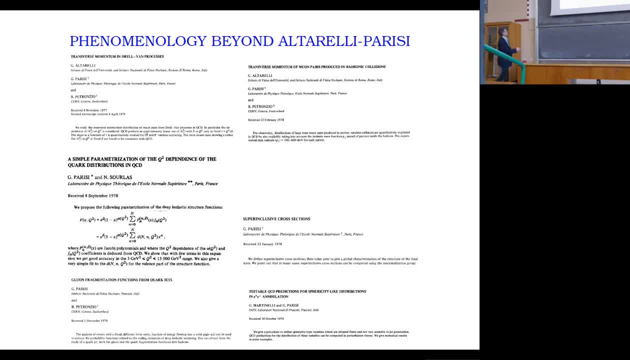 which is defining what we call the jet C parameter and sphericity glue and fragmentation from quark jets and again sphericity like distribution. So a number of developments which we would call modern jet physics. Let me just go quickly through a couple of these developments. 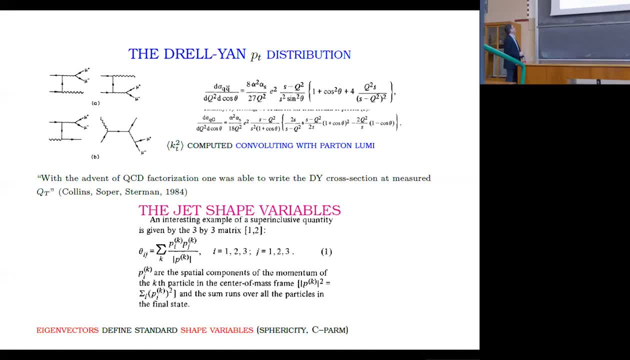 to give you the flavor of them. One has to do with Drellian, where this is a paper written, this one written in collaboration with Guido and with Roberto Petronzio, where the PT distribution of Drellian pairs in what is currently called the Collins-Soper frame. 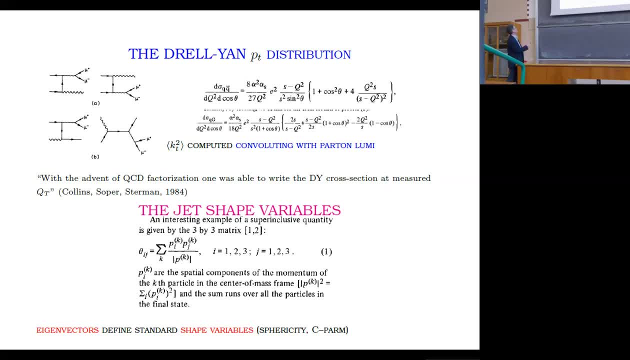 is computed, and in the famous Collins-Soper-Sterman paper of 1984, where they do for the first time the modern version of PT re-formation, to next to leading law, they say, with the advent of QCD factorization. 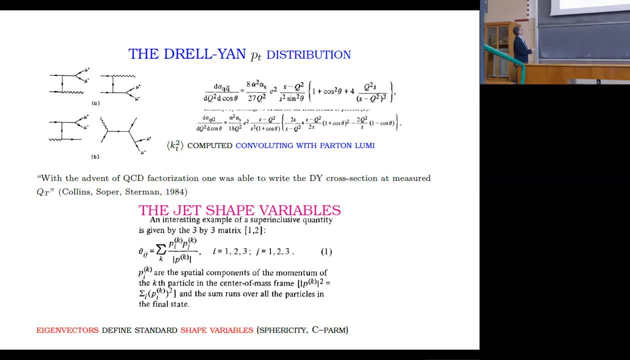 one was able to write the Drellian cross section at measured QT and then they give it as a reference, this calculation. So you know this was recognized as the birth of QCD factorization, The other paper I'd like to mention. 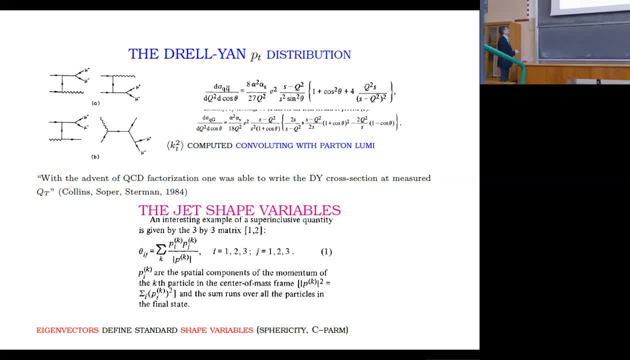 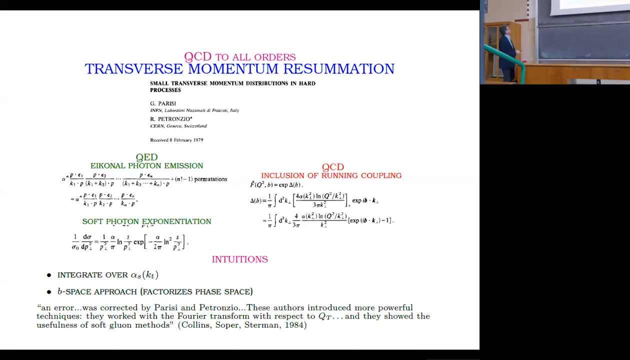 is the one on, you know, super inclusive variables, where one defines this quantity, which is a tensor whose eigenvectors define theance, the modern shape variables, the sphericity, the C parameter, the spherosity, and so on. 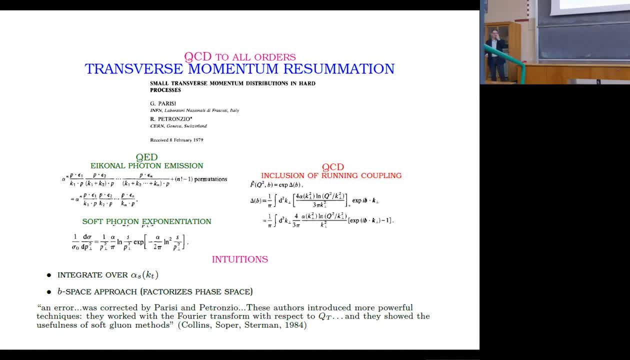 Now I'd like to spend my last five minutes or so by briefly mentioning a final line of development, which has to do with trying to go beyond fixed order perturbation QC. Now, of course, much of the work that Georgia was doing in these years had to do with the high order behavior. 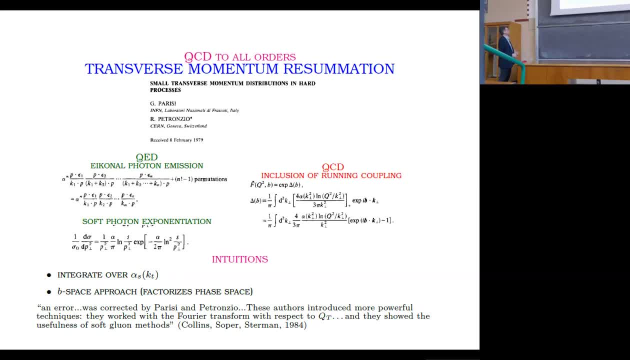 of field theory in general. But you know, a related line of thought was: are there aspects of perturbative QCD calculations that we can perform to all orders? And there are at least two seminal papers in this respect which have to do with what we'd modern in modern language. 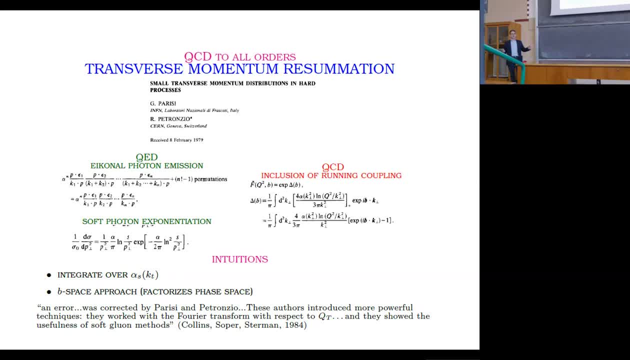 we'd call pseudocompressorimation of PT distributions or, of you know, threshold, pseudocompressorimation of soft logs. Now, these two papers I'd like to spend a few minutes about, because both of them contain some interesting and surprising insights. So the first paper, which is quite 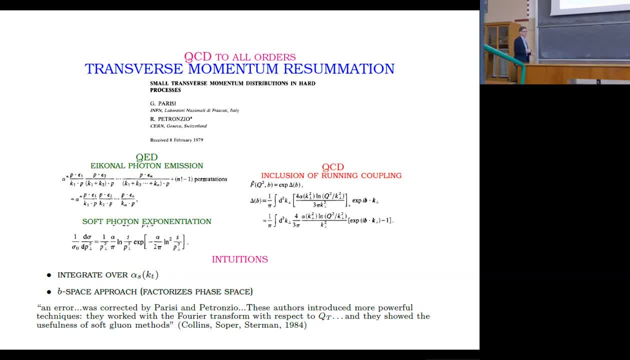 famous. I guess many people, many practitioners of perturbative QCD know it. I knew of it. It was written together with Roberto Petronzio And it's the first paper in which transverse momentum resumation is included. This is something which is very important because at small PT, 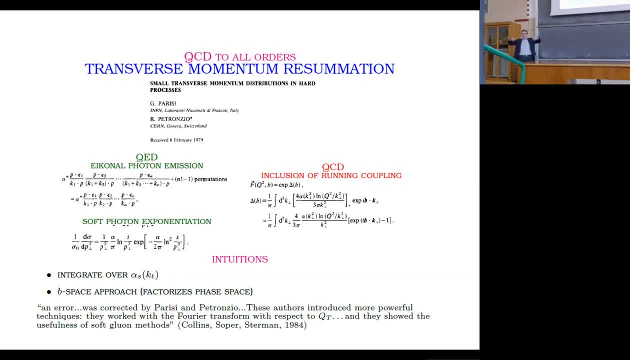 a fixed order calculation produces divergent results, while if you sum to all orders you get a finite result. So you're forced, if you want to compare to data at small PT, you're forced to perform this resumation In this paper. this is first done in QED by using the icon approximation. 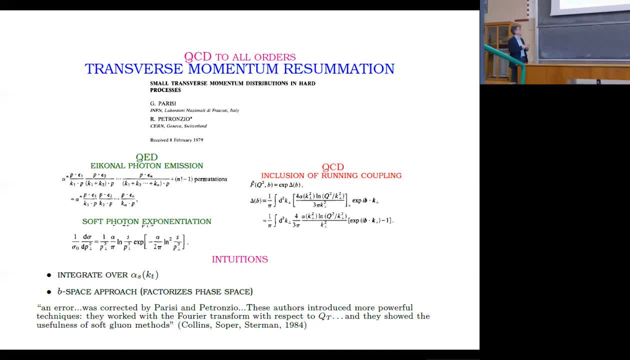 for soft photon emission and then including running coupling effects to move towards QCD. And you know there are a couple important insights here. One is that the running coupling effects are included or resumed correctly by letting the coupling run with the KT which you 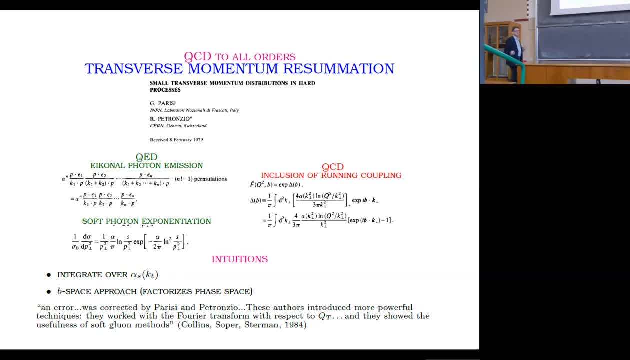 are integrating or resuming upon. And the second insight is to use a B-space approach. So take the Fourier transform. and that's because, if you're doing a transverse momentum distribution, taking a Fourier transform factorizes the phase space, The delta. 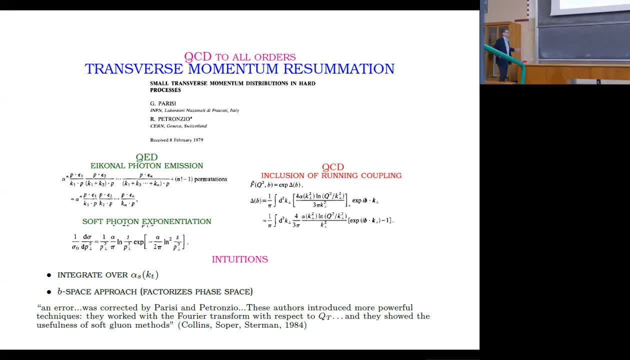 function that gives you transverse momentum conservation gets factorized and then you get immediately the result. And in the same Colin Soper-Sterman paper which systematized and produced the modern version of this, you know they say that the previous error by the Russian, 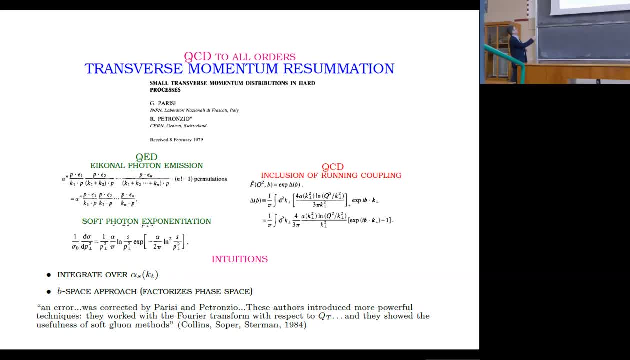 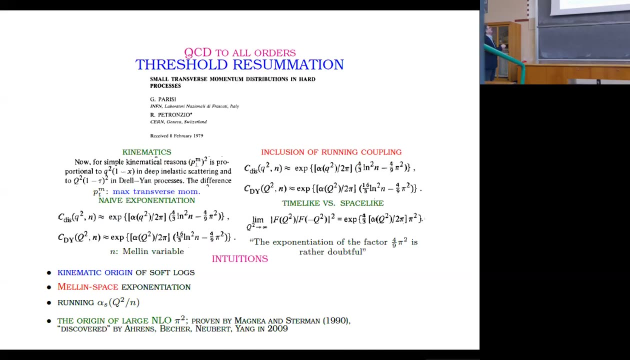 school was corrected by Parisian Petronzio. this paper, These authors introduced more powerful techniques. They worked with the Fourier transform with respect to QT, and they showed the usefulness of soft gluon method. So this is really the origin of modern CSS as it is currently known. The other paper is about threshold resumation. 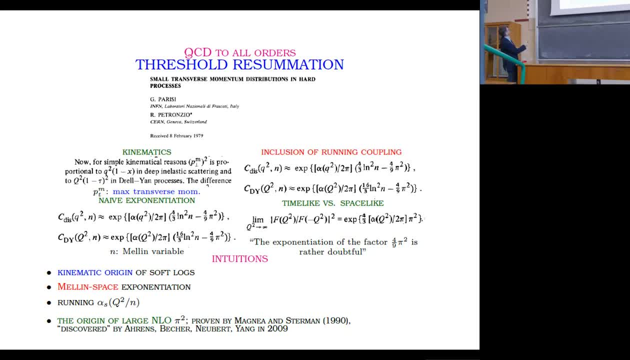 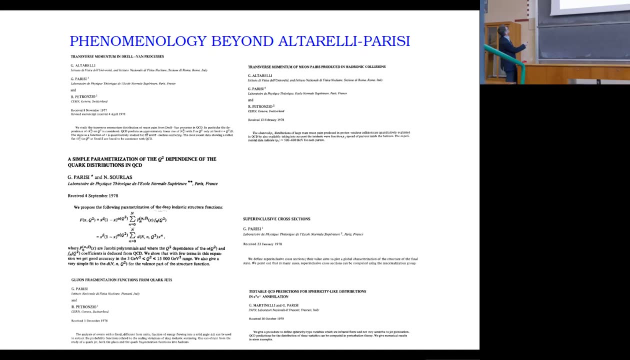 I guess. so here. I'm sorry I put the wrong. yeah, So apologies, this is not the right citation. The right citation would be the paper down here, the paper, okay, no, okay, sorry, So I missed the right paper. It's a paper. 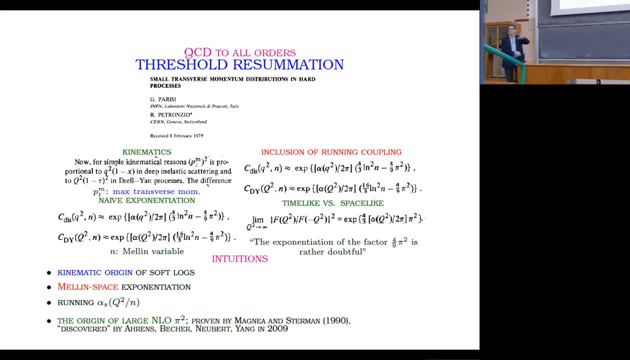 which is written by George, a single author. I'll replace this in the slide you can put on the website Now. this paper does not perform the resumption of PT, but rather resumption of the total center of mass energy for processes like Drellian, or in modern language, or in: 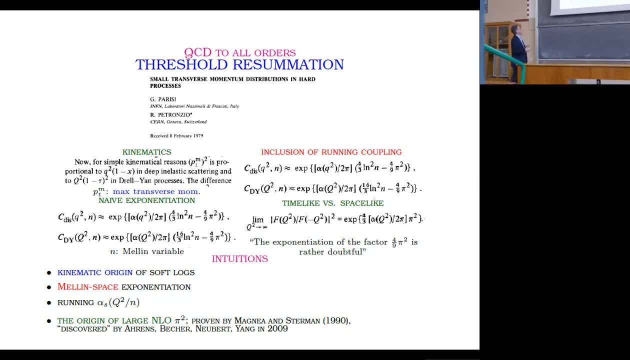 modern days, Higgs production, and it contains at least four very important insights. So the first important insight is that resumption- soft resumption- has a kinematic origin and it has to do with the fact that the maximum value of the transfer of momentum is driven by a quantity. 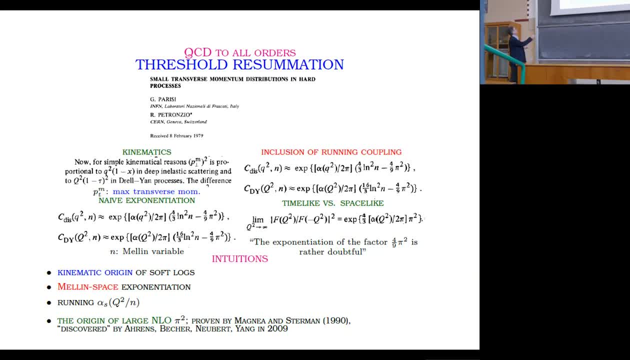 which is related to a soft scale. So it's a hard scale Q-square multiplied by something which is one minus x in de-binastic scattering, one minus x in de-binastic scattering and one minus x in square in Drellian. So when x goes to one, this hard scale becomes a soft scale, and this is what 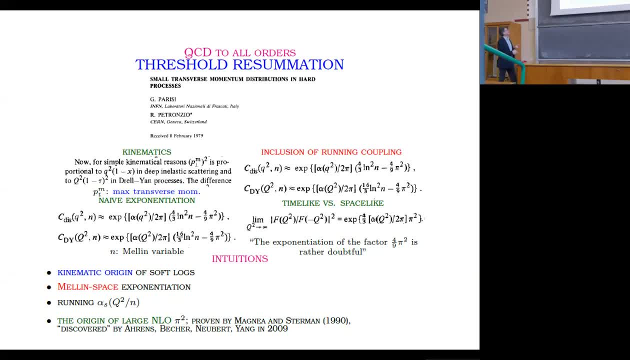 you're resumming. The second insight is that running coupling effects are included by letting the again the strong coupling run with the soft scale. and the other important insight is that the resumption is best realized by taking an integral transform which is now no longer a. 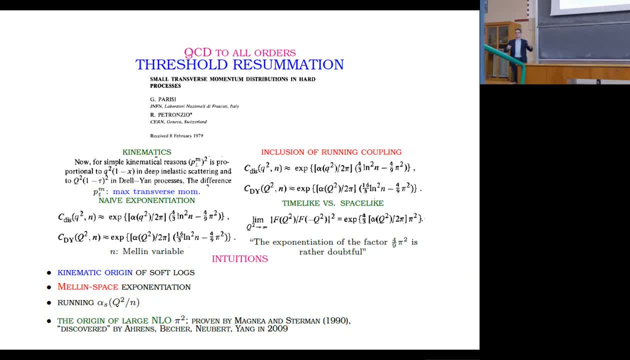 Fourier transform, but rather a Fourier transform. So the second insight is that the resumption is best realized by taking an integral transform, which is now no longer a Fourier transform but rather a Mellin transform, because Mellin decouples longitudinal momentum like a Fourier decouples. 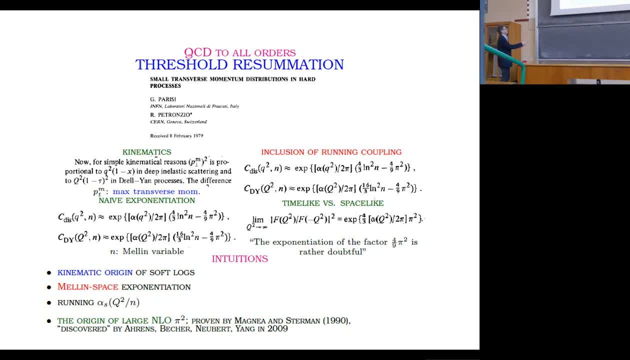 transfer of momentum conservation. And the final interesting intuition is a relation between DIS and Drellian resumption, and particularly the fact that in the large Q-square limit the ratio of DIS to Drellian is driven by an analytic continuation of the logs from: 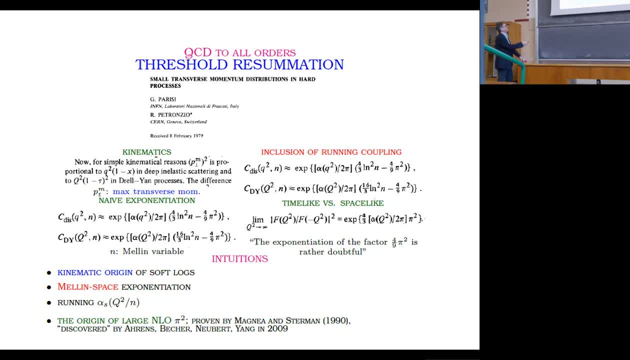 spacelike to timelike, which produces pi-square. you know you have a, you know you have a pi for each log. they are square logs, so you have pi-square factors and then you get an exponentiation of pi-squares which Giorgio describes as being rather doubtful. of course. 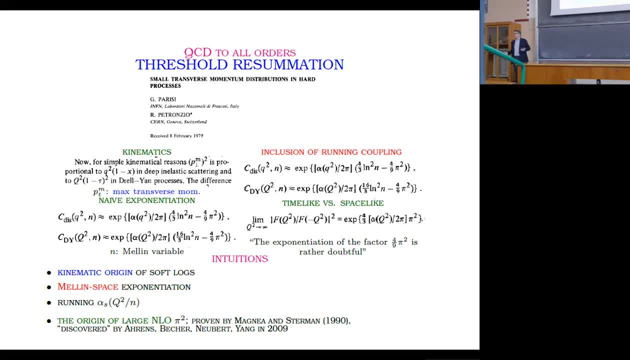 because you know you're exponentiating constants which are there, but of course there are other constants which you're not exponentiating and which are not universal, and the constant is a constant, it's not like a log. Now this last exponentiation of constants was rediscovered. 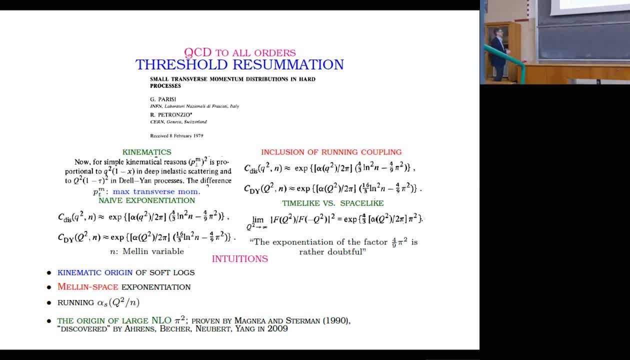 several times. It's actually proven by George Sturman and my friend Lorenzo Magnea in his PhD thesis in 1990, and then there is a paper by our SCET friends Matthias Neubert and collaborator, who claimed a huge, important discovery in 2009,, exactly 30 years after this paper was written, where they discover: 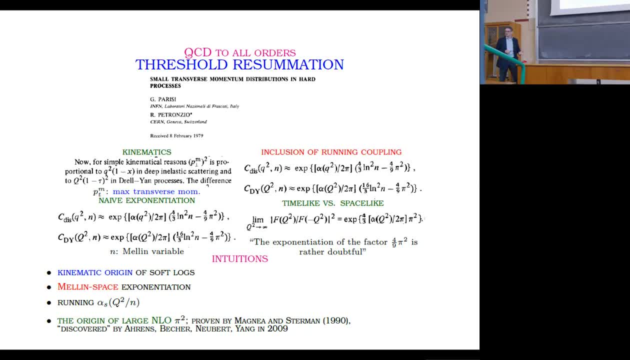 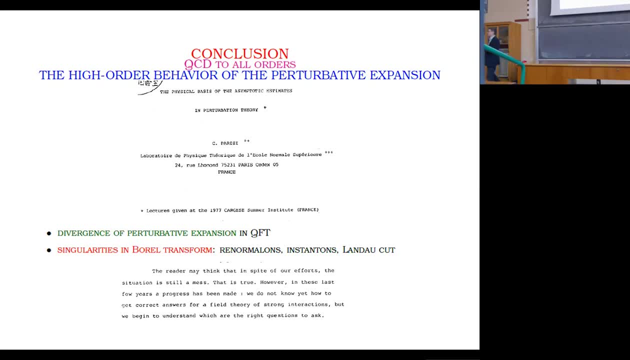 this equation here and they, you know, present it as a major breakthrough. So this brings me to the end of my talk. This idea that you could look at the all-order behavior of perturbation theory was clearly something potentially interesting and something that might go beyond perturbation theory, and Giorgio worked a lot. 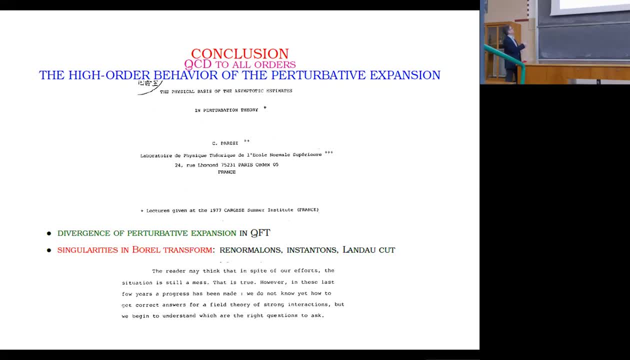 on trying to study the asymptotic behavior of perturbation theory in field theory by studying the diversions of the expansion of field theories in general, gauge theory in particular, studying their Borel summations, singularities and the Borel plane, and in these lectures from the late 70s, when coming to gauge theories and 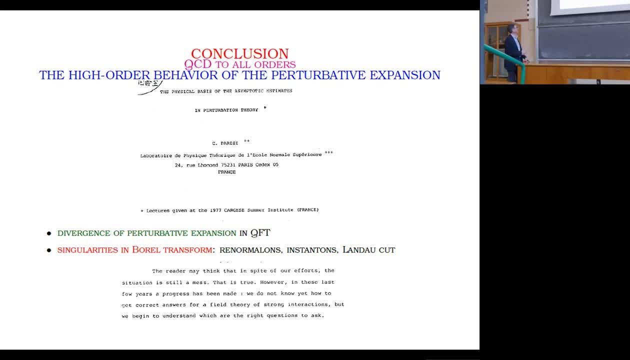 QCD Giorgio concludes saying: the reader may think that, in spite of our efforts, the situation is still a mess. That is true. However, in this last few years of progress has been made. we do not know yet how to get correct answers for a field theory of strong interactions where, here, by correct, 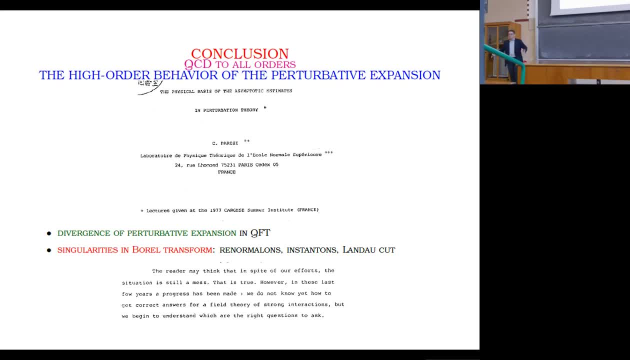 answers. what he meant is, you know, non-perturbative QCD, basically. But we begin to understand which are the right questions to ask. This is one of the last QCD paper, or perturbative QCD paper, that Giorgio wrote, and then he: 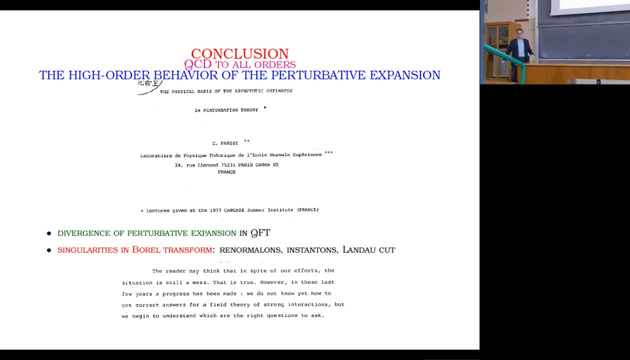 obviously thought that the way of actually answering these questions was by using the lattice, and that is the subsequent line of development, which someone else will be talking about, and therefore I'm going to stop here. Thank you very much. Okay, thank you very much, Stefano. It was a very, very nice seminar. Do we have questions? 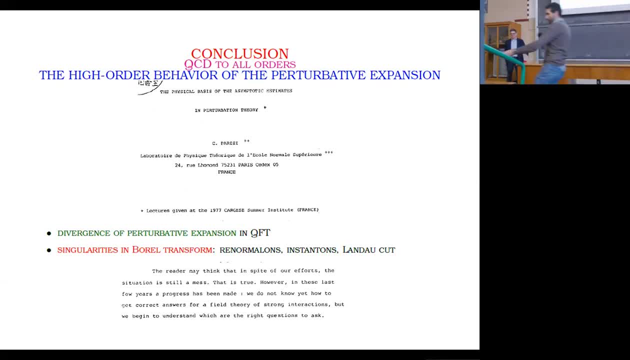 Ah yeah, If you want to. Well, first of all, I would like to thank Stefano for this wonderful, very careful reconstruction, and I would like to add something which you could not probably know: that Nicola Cabibbo was the one that stressed the importance that was both Tisci's advice on myself and 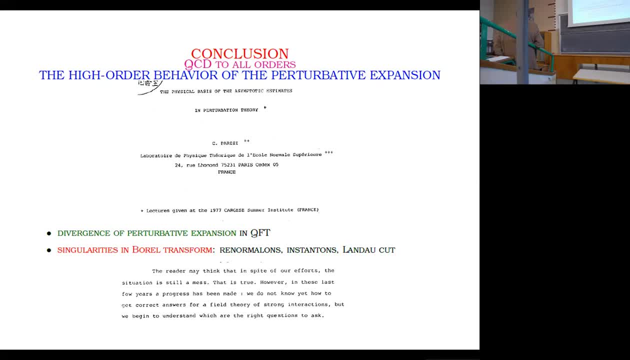 also of Francesco Givilli, stressed the fact that by taking Williamstein pre-computation- because he was doing with taking Williamstein computation for some processing in a plastic binocular, and also of Linus Theodone, other processes, and indeed he pushed us to write down the 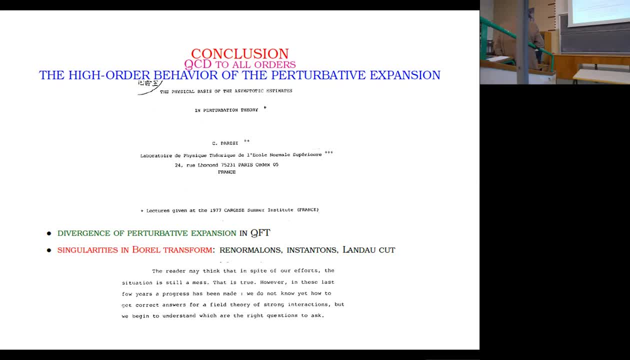 licit amplitude and so on. And also the point is that before the Altavelli-Pervisi paper there is a nice, very nice paper, which unfortunately is only a CERN pre-print, unpublished, of Cabibbo and Rocca. 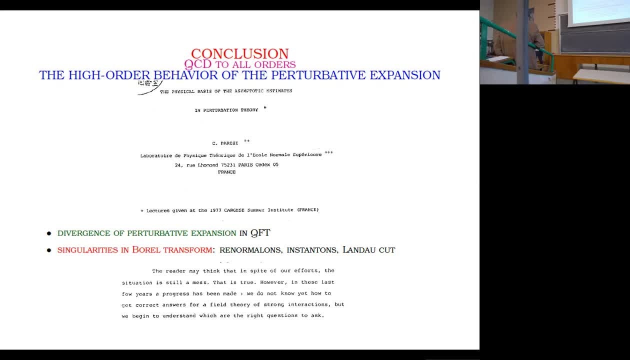 Cabibbo was the thesis advisor of Rocca for CERN. For some reason the paper was just only a CERN pre-print, in which they were doing the computation in electrodynamics of the splitting function in the P-infinity limit. 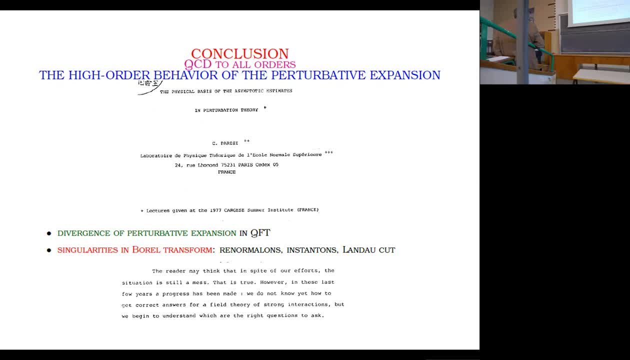 So the idea of using the P-infinity limit is something that Nicola pushed strongly because he liked it very much. and he did not only that, but take Williams in the P-infinity limit, which probably you could find in the text or it was done by other people. 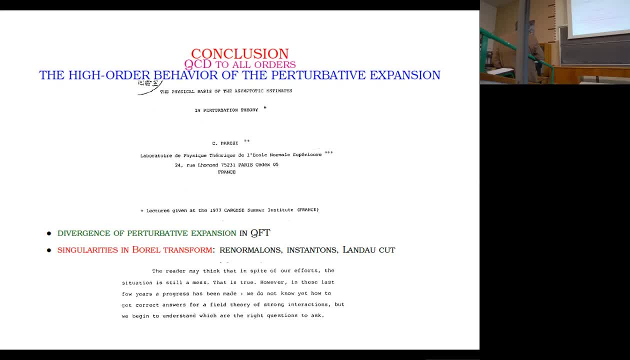 But he also computed the splitting function for a photon going in a plus and minus pair. So of all the three splitting functions that we need, the only one that was missing essentially in the Altavelli-Pervisi was the Grouin-Grouin-Grouin splitting function. 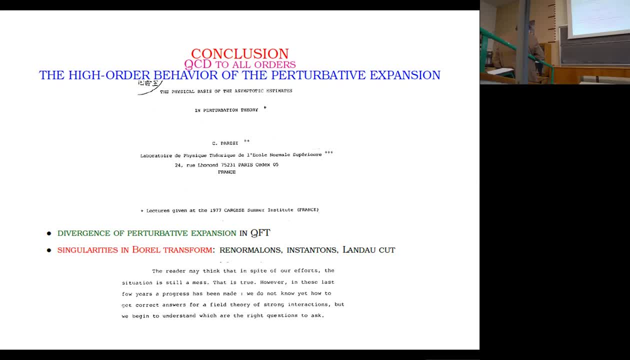 The other things. one difference, an important difference that fortunately people do not realize between the Morion lecture note and the Altavelli-Pervisi paper, that some of the formulas of Morion are wrong. There are some mistakes, which maybe I was. 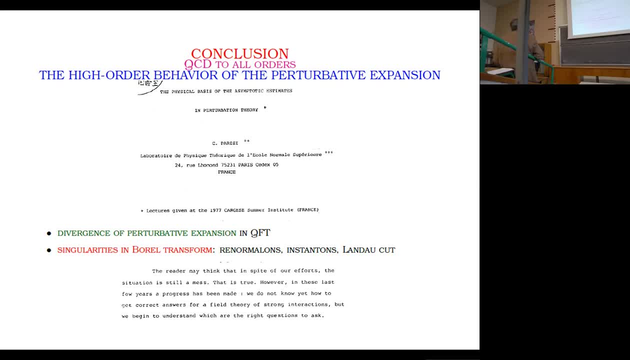 Well, there are some mistakes. One of the things, something that should be symmetric, was not symmetric, so there are some x's place one minus x, and so on. Okay, thank you, Thank you again, Thanks. Questions from the audience. 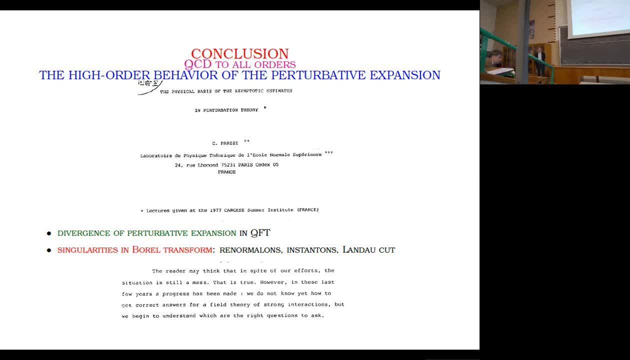 Comments. Just a curiosity, because I was used to associate the jet shapes to fragmentation models, because I was working on that many years ago, 40 years ago, And I didn't know the contribution by Giorgio Parisi, Which result he obtained and how do they compare with experiments? 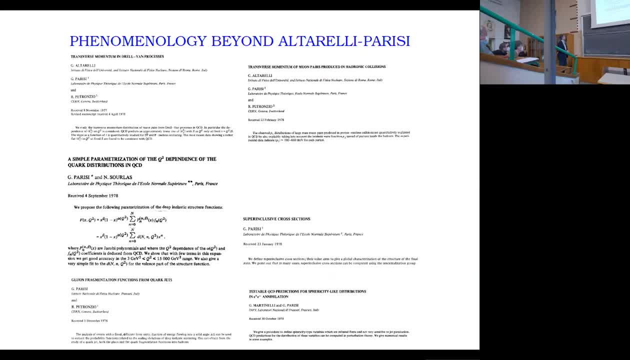 if you have some information, So indeed I could look. Well, I guess maybe Giorgio can answer better than myself. I could locate three papers of Giorgio on jets. One indeed is Grouin fragmentation function from quark jets. 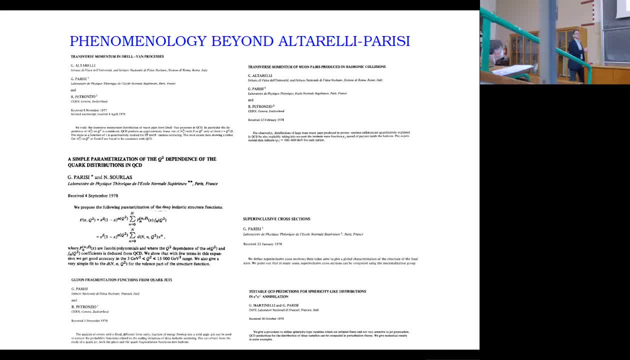 which is using fragmentation models, But the other two are actually defining what we would call, in modern language, jet shape variables. So one of the two defines a generalized. So this is a testable QCD prediction for sphericity-like distribution. 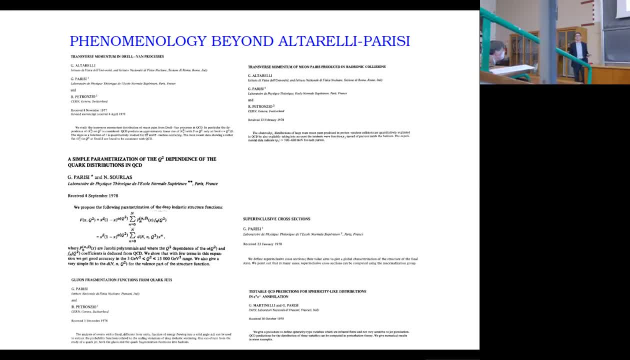 So it defines a generalized sphericity which includes what we would call spherosity in modern language. You may know that the original sphericity was not infrared collinear safe And in this paper, you know, the sphericity is generalized to a general exponent. 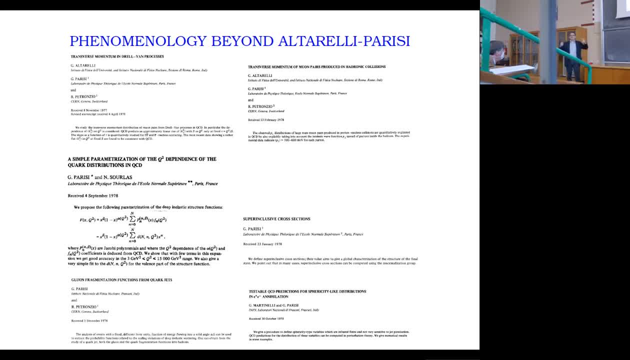 in the momenta in the numerator, such that for one particular choice you actually get the infrared collinear safe variable. And the other, which maybe is even more important, is this paper called super-inclusive cross-section, where he says: we define super-inclusive cross-sections. 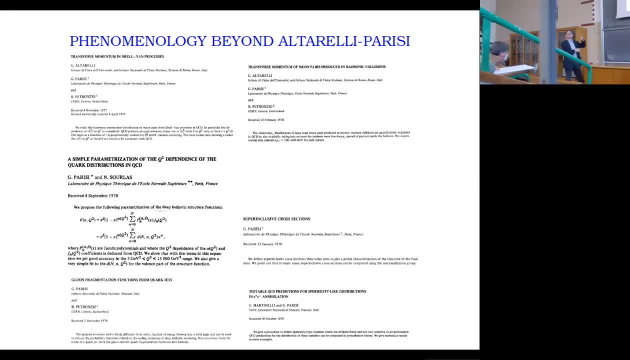 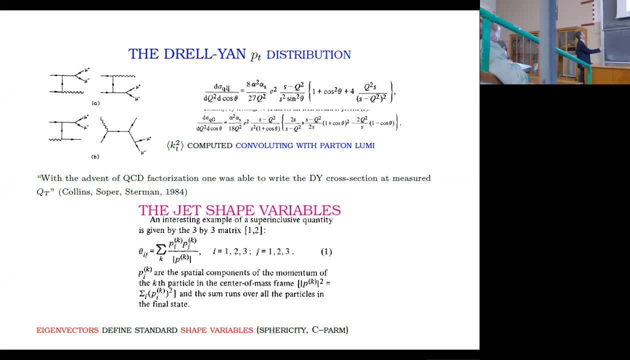 which you know, it's something which is more inclusive than the cross-section itself, And so an interesting example of super-inclusive quantity is given by the three-by-three matrix, which is this And this guy here. if you look at the eigenvalues of this matrix, 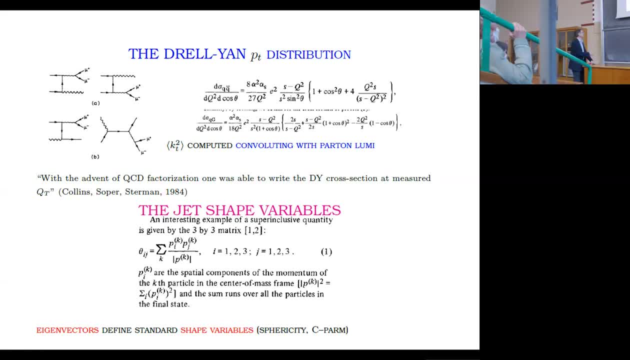 which is sometimes, still today, called the Parisi matrix. then you realize that one of the eigenvalues is what is called the C parameter, The other is the sphericity, And so you have this tensor here, constructed out of the momenta of you know. 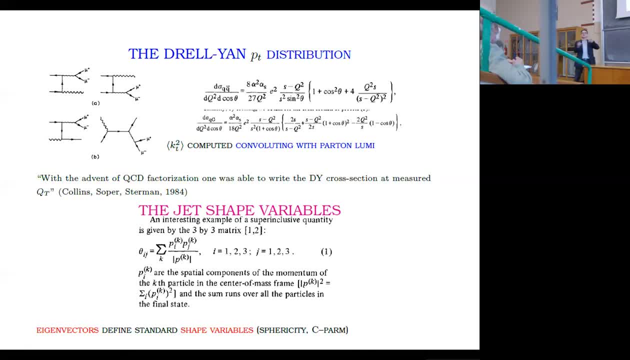 PIK are the spatial components of the momenta of the kth particle in the center of mass frame. So out of the momenta of the outgoing momenta of the outgoing particles, you construct a jet-shaped variable which is, you know, the modern jet-shaped variables. 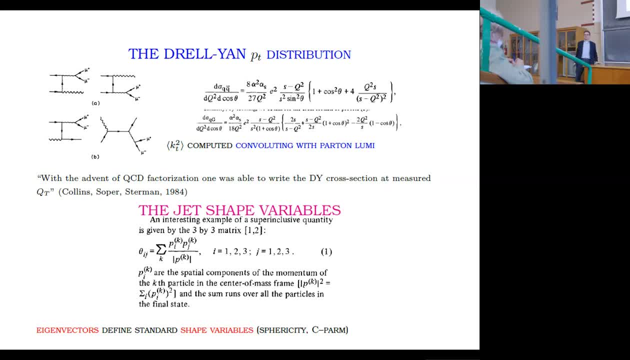 So this is like the, you know, the ancestor, the progenitor of a number of modern jet-shaped variables. So this is not a fragmentation function, It's just a shape variable. So, for example, it's the kind of thing that people today 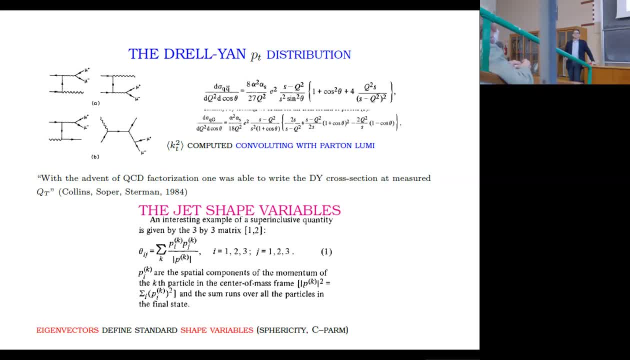 use to tell a quark jet from a gluon jet. Other questions or No, Maybe? just if I can add this: I became aware of this the other day by discussing with my colleague in Milan, Giancarlo Ferrera, who is teaching a course on the standard model. 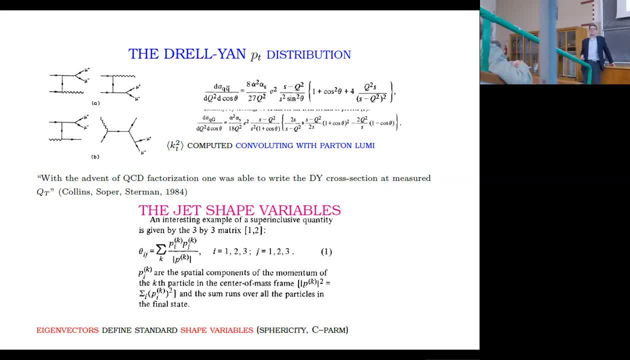 and he was using some notes given to him by Stefano Catani, where in the notes by Catani there is this expression, and he said: well, this was originally proposed by Parisi. Okay, no, I was just thinking to Stefano Catani. 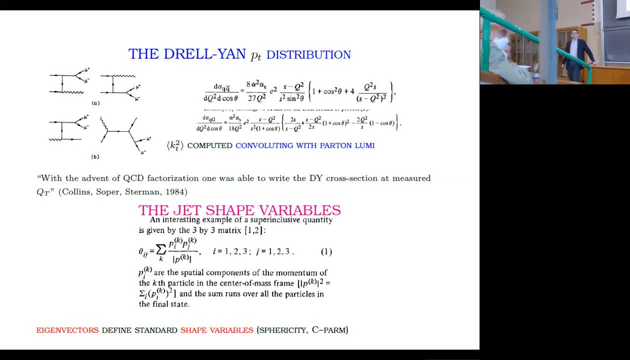 he was doing something like that some 30 years ago. Yeah, yeah, of course, This was then developed in the 90s, basically when people at Hera started doing Hera jets. Well, if there are no more questions, I think we can thank Stefano again. 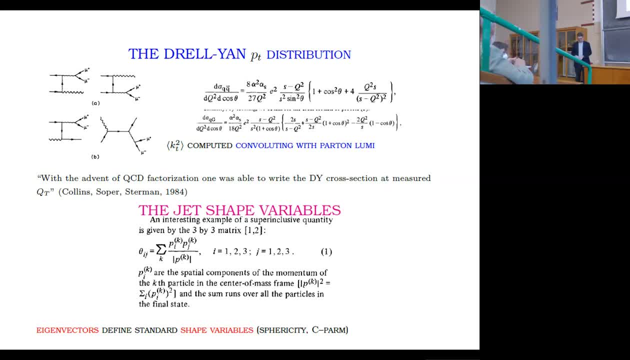 Thanks very much, And we now have a coffee break outside so you can go and eat and drink.